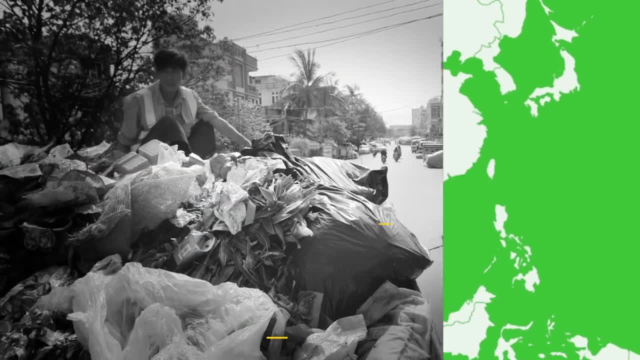 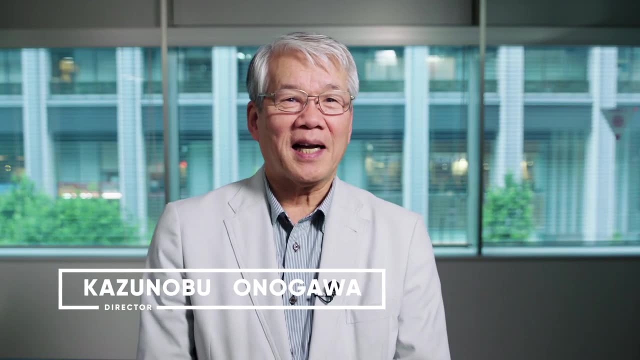 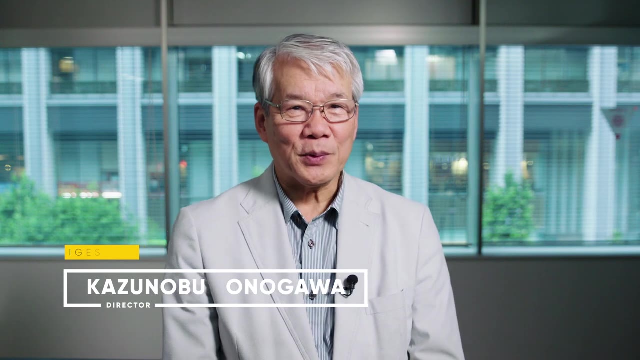 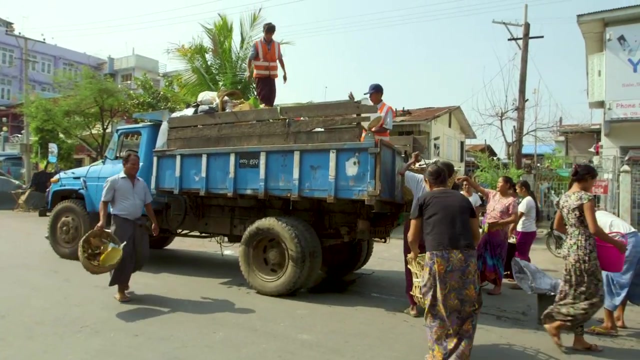 country. This is a case study to illustrate each step of the process. In most developing countries and their cities, waste management is limited to waste collection and disposal. The aim is to collect as much waste as possible to keep streets and neighbor foods clean. 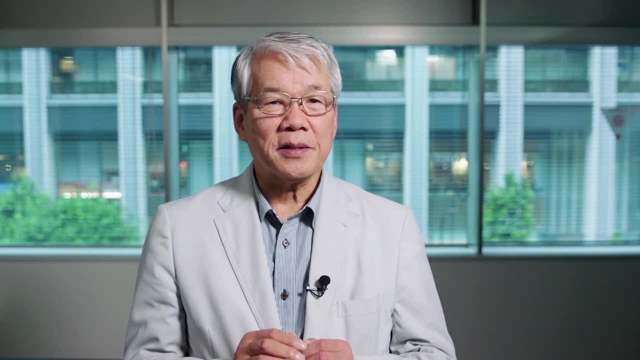 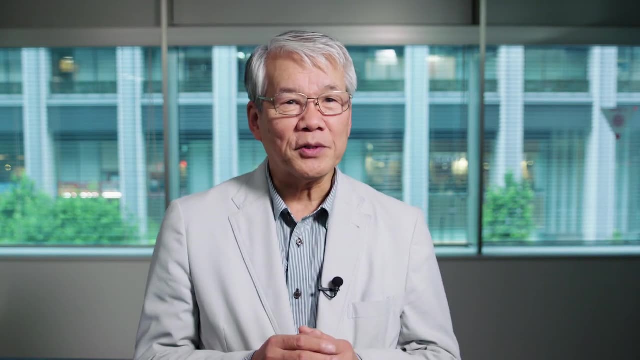 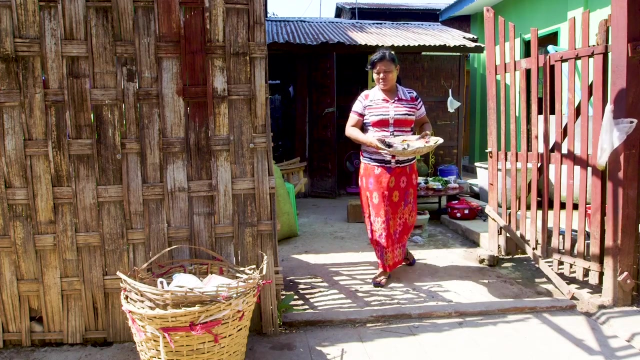 However, these countries and cities are辛가, as we call them in Mandalay mean waste collection and disposal. cities never seem to have enough capacity and infrastructure to deal with the growing amounts of waste, Even when collection keeps up with the growing amount of waste we are. 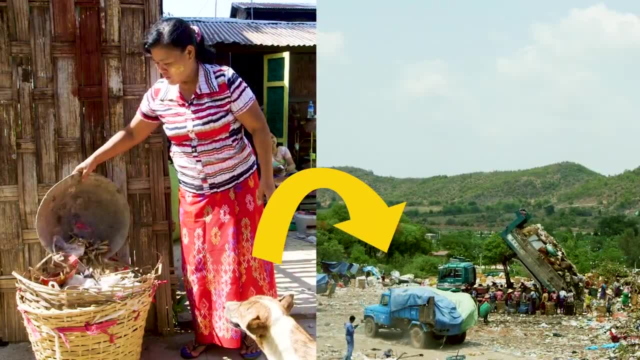 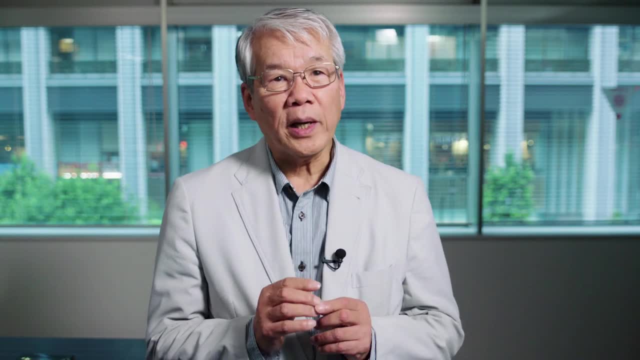 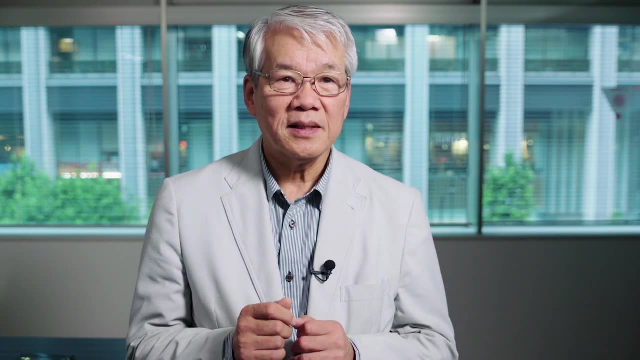 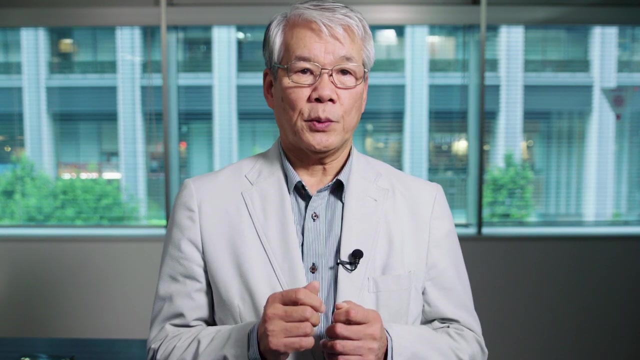 just transferring the problem from the streets to landfill sites or some other location. We propose a shift in the way we look at this problem. We should see waste as a valuable resource. If recyclables are separated at home, for instance, they can be sold generating 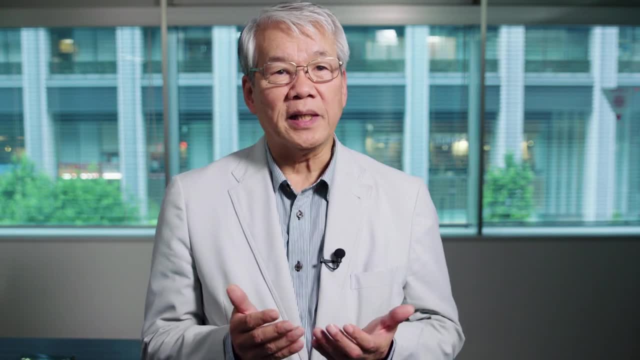 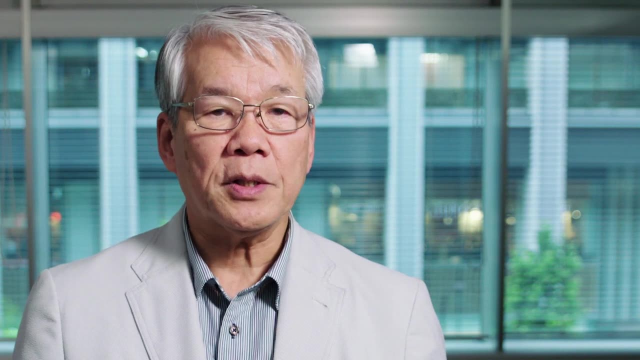 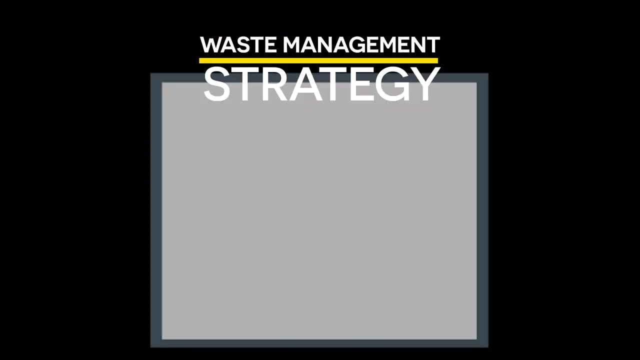 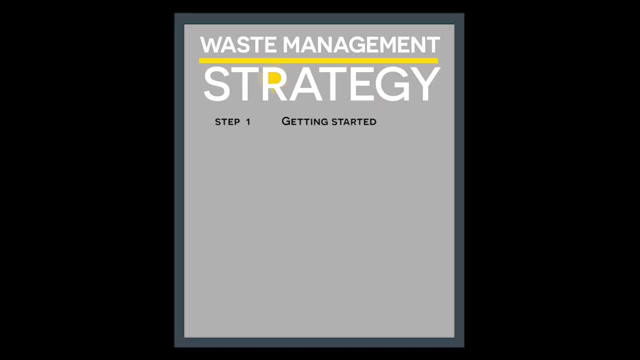 income while keeping our environment clean. To best consider solutions in the context of the waste management system you want to improve, a fundamental first step is the development of a waste management strategy. The strategy is a roadmap that will guide the team leading the process and the many stakeholders involved. 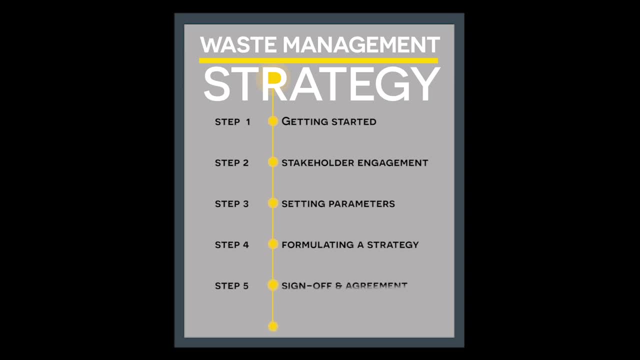 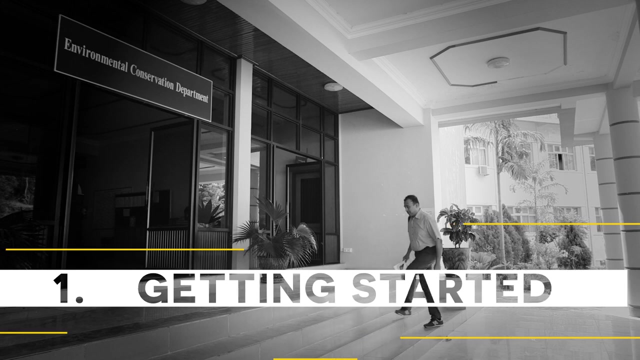 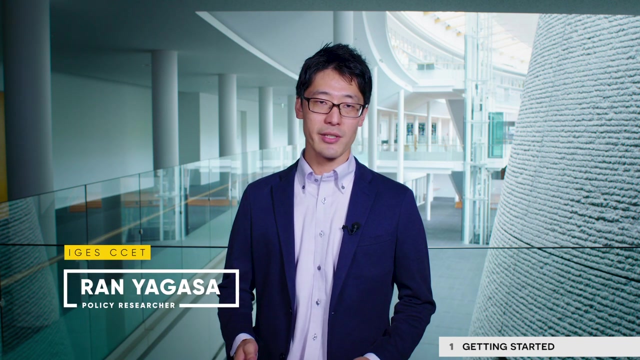 to come up with appropriate solutions for the local context. The waste management strategy development process consists of six steps. Step 1. Getting started. Each country or city will begin this process from a different point, but the essentials for everyone include a number of elements. 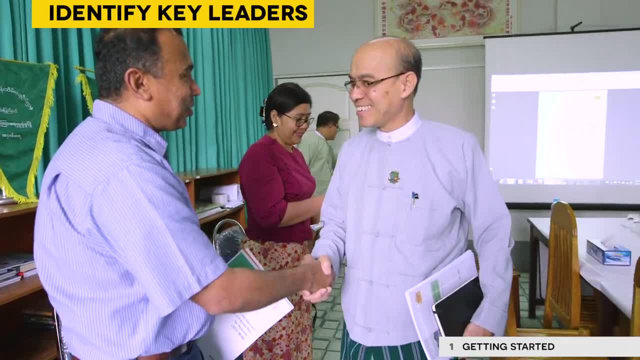 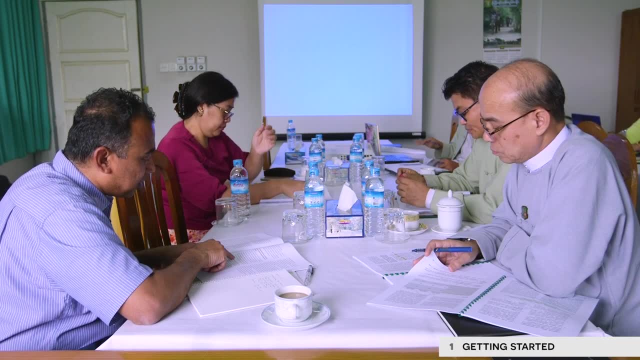 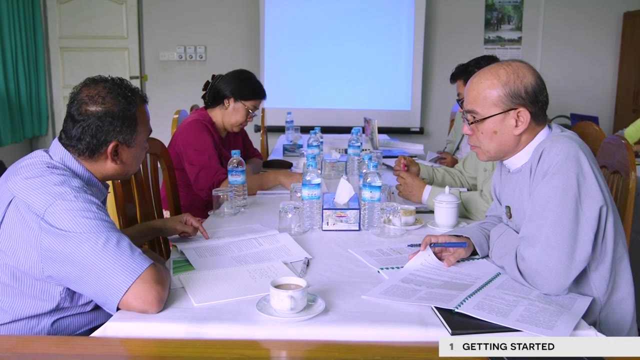 Identifying key leaders. Identify and engage with the key government agencies dealing with waste. A person or group in the political leadership must be selected to be in charge and given the responsibility to manage and deal with waste. A group of people in the for driving the waste management strategy process. 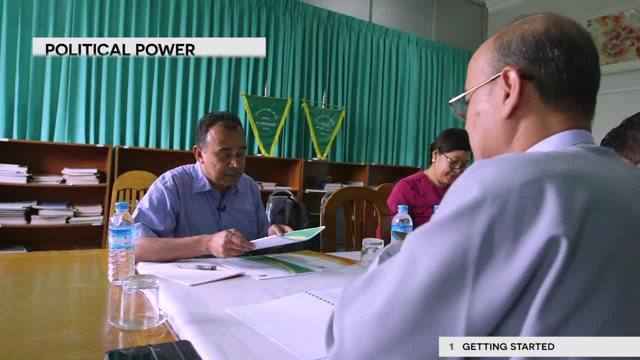 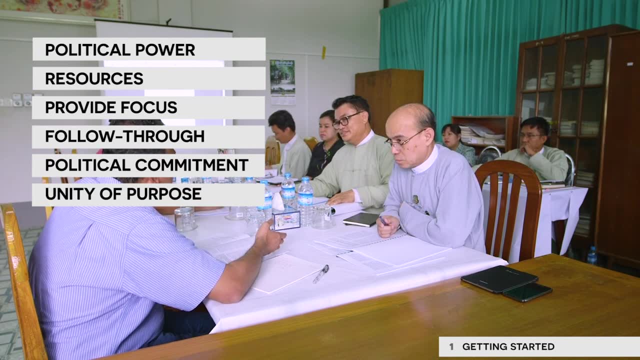 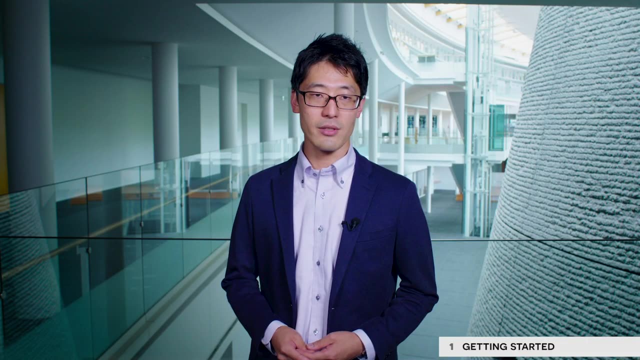 The organization that takes the lead should have the political power and resources to provide focus and follow-through, providing political commitment and unity of purpose. Officials will need to be assigned to support this project and are likely to need resources such as a project office, budget and workforce. 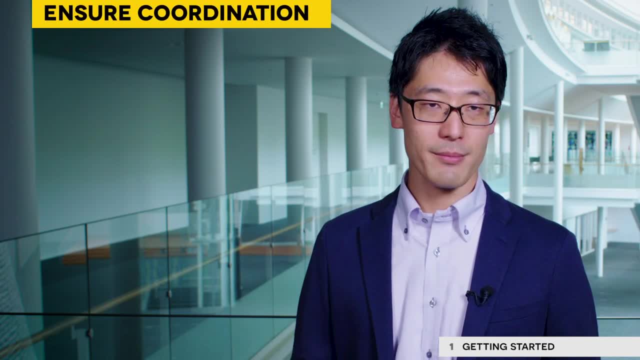 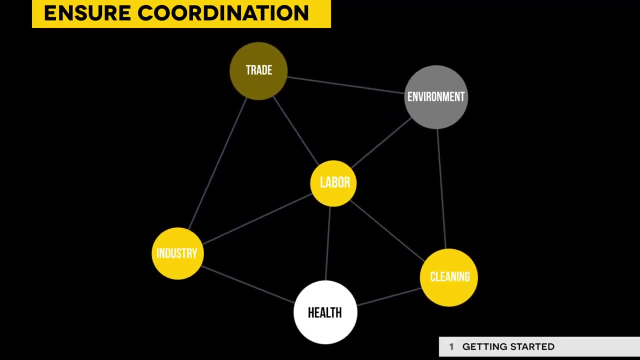 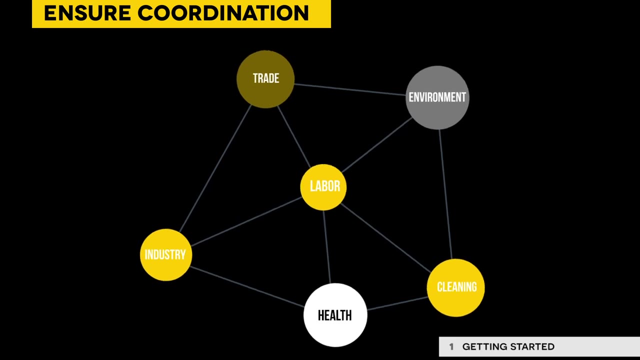 Ensuring Coordination Mechanisms. Different aspects of waste management are often the responsibility of various government agencies, so it is important to have internal coordination among all of them. This will ensure all relevant parties are aligned with and actively supporting the development of this strategy. 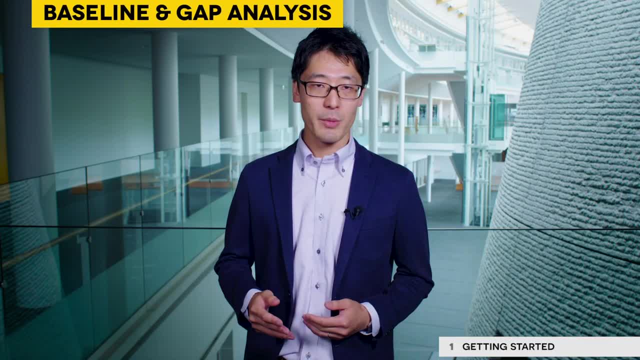 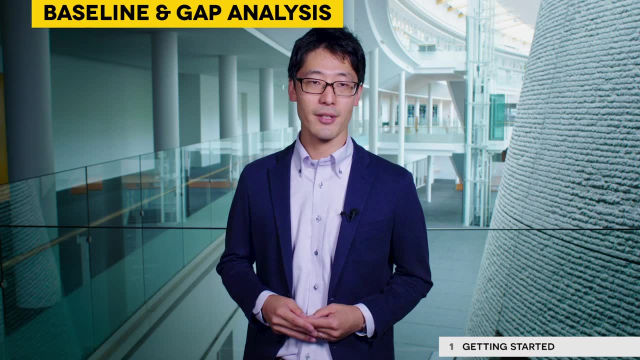 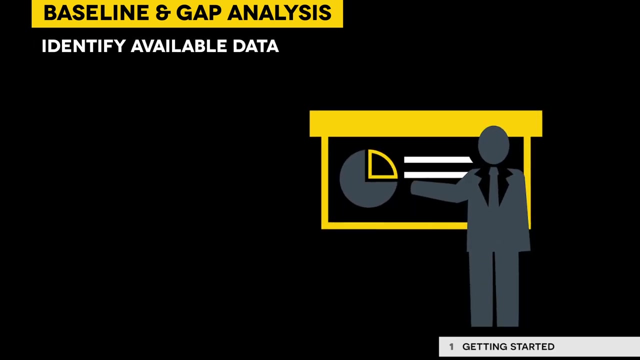 Baseline and Gap Analysis. Determining the current situation and how well the waste is being managed is central to developing a useful strategy. The following steps are important for understanding the current local situation and identifying the gaps that need to be addressed: Compile all waste-related data available, including information on waste generation. 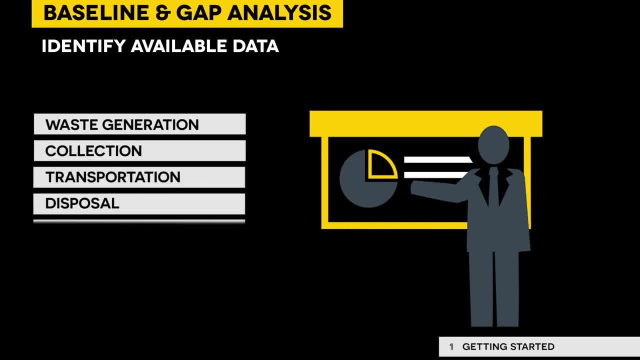 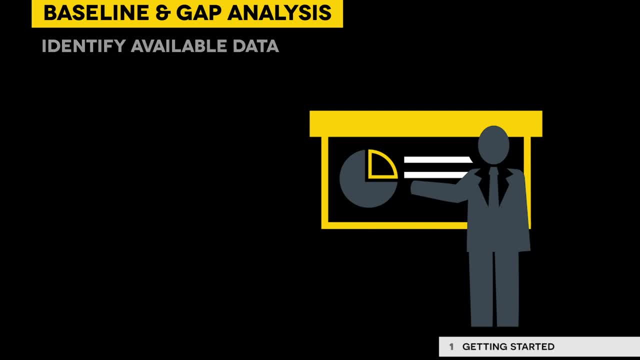 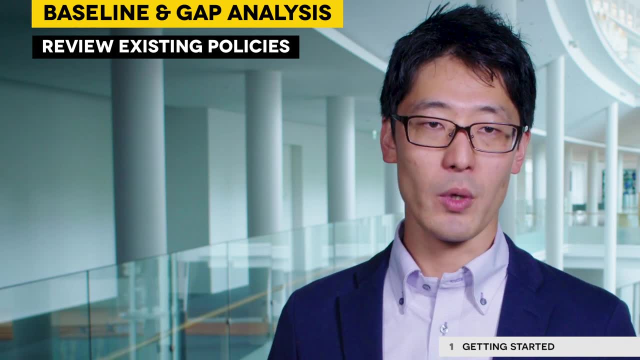 collection, transportation, disposal, waste classification and composition. If data is not available, surveys and sample studies may be needed. You need to review waste management policies currently in place so you understand the current waste management system and how the new waste strategy is going to be interlinked with existing policies. 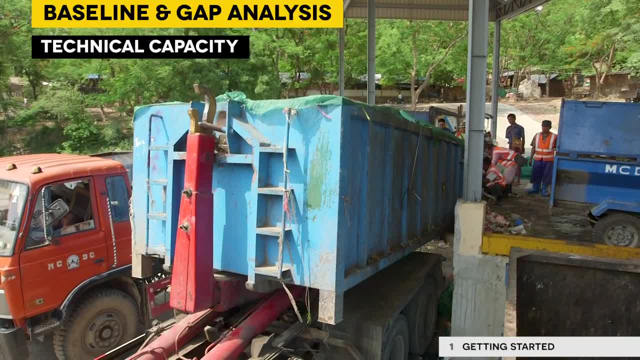 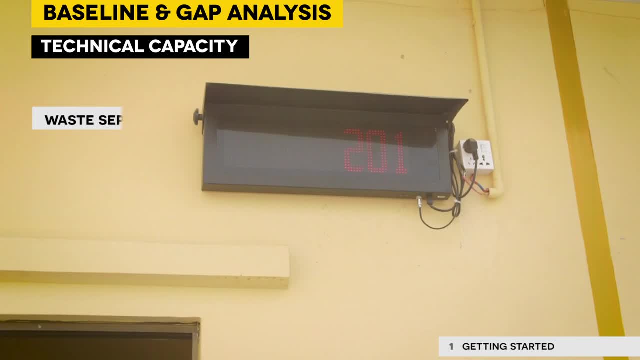 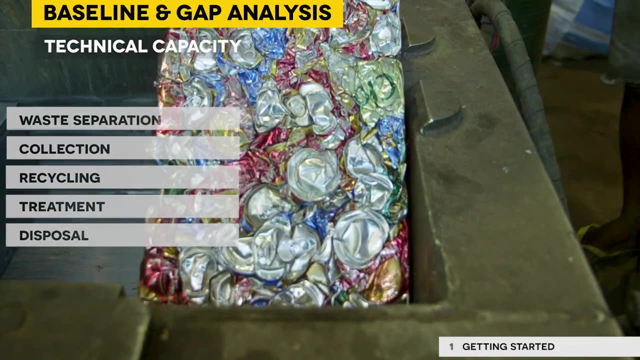 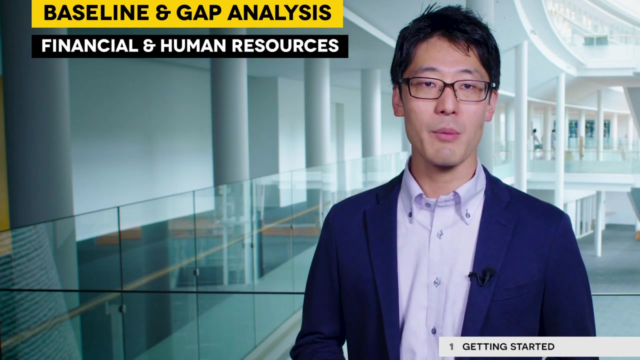 Develop an understanding of the technical capacity and infrastructure available in the city or country. This technical capacity can be related to waste separation, collection, recycling, treatment or disposal. Financial and Human Resources. Financial and human resources will be needed to implement improved waste management practices. 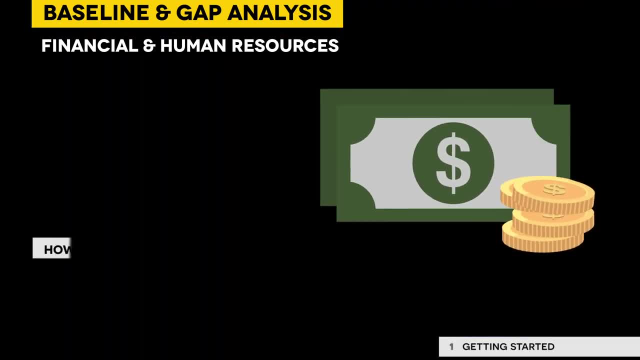 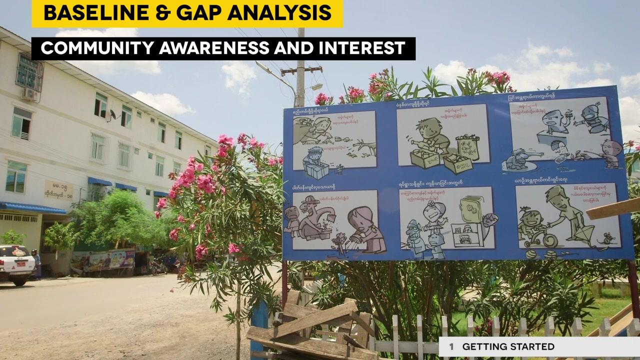 so develop an understanding of the resources available. How is waste management currently funded? Are there cost recovery schemes in operation, through taxes or fees? Are the resources adequate? What technical skills are available? Consider community awareness and interest. This strategy will call for public participation in the planning and implementation of initiatives. 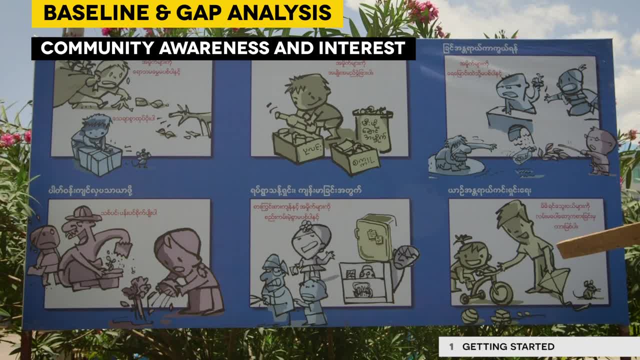 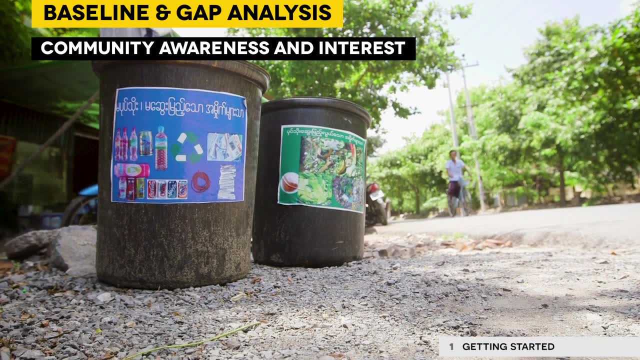 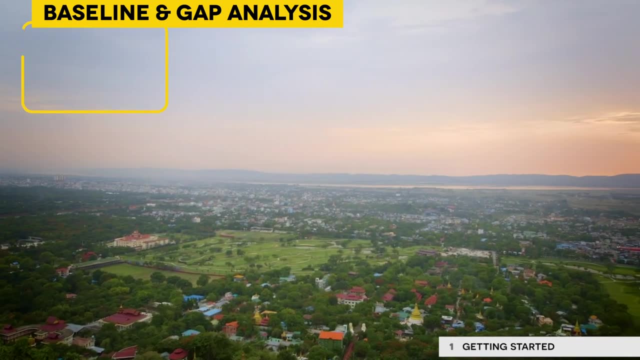 People may be requested to separate their waste or use special waste bins. For this reason, it is important to understand the level of awareness regarding waste management among members of the public and private sectors and the community. In Mandalay, IJS CCT. in cooperation with the Government of Myanmar. 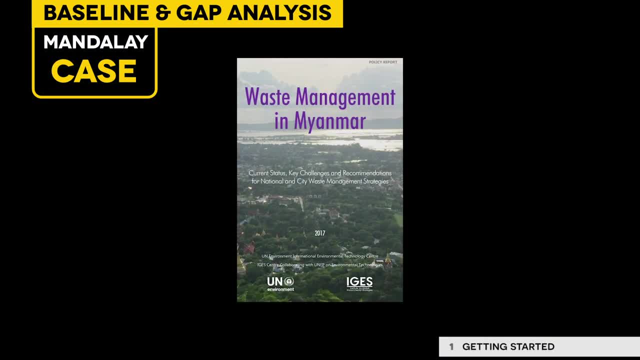 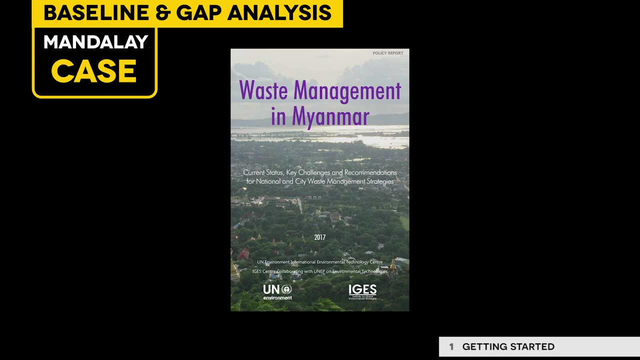 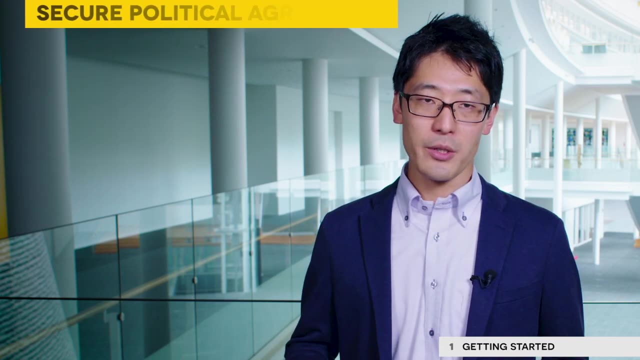 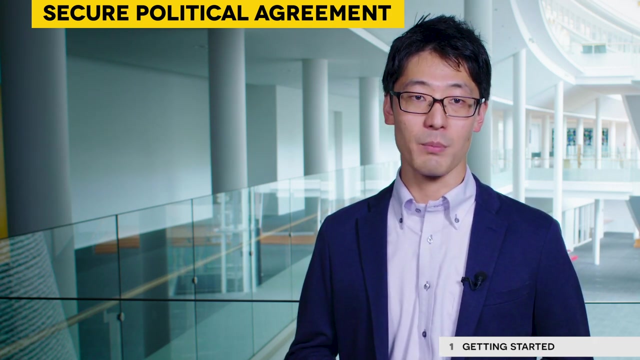 published the policy report Waste Management in Myanmar, providing the findings of the situation and gap analysis, supporting informed decision-making towards the creation of the waste management strategy. Secure political agreement: Create an initial agreement with relevant agencies showing the approval and commitment of political leadership with the development of the waste management strategy. 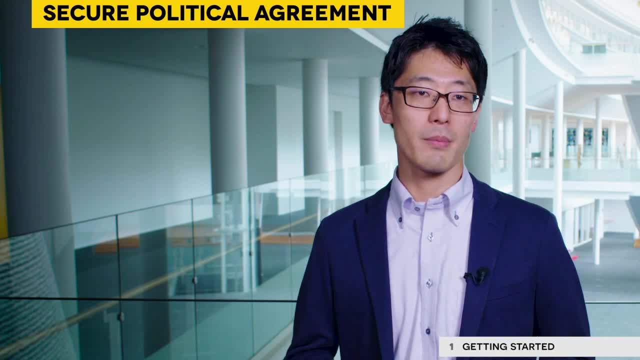 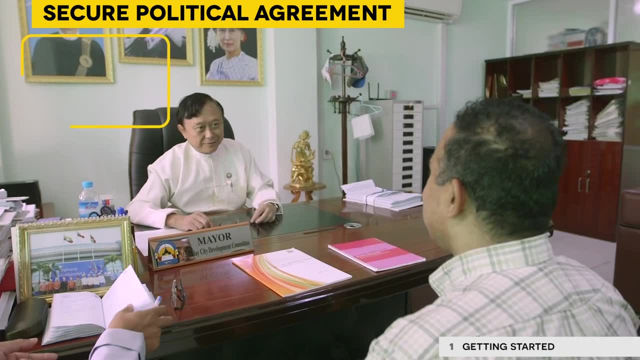 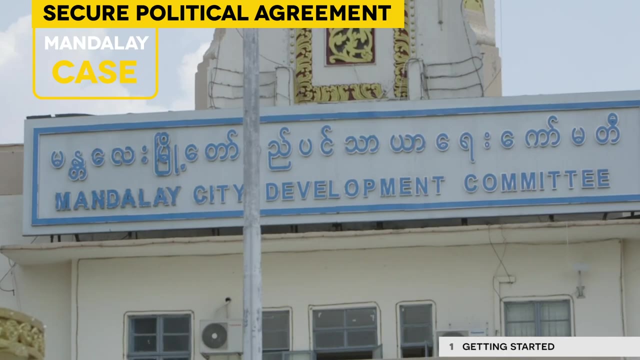 At the city level, this would preferably be the mayor. In the country case, it should be the relevant minister. In the case of Mandalay, the IJS CCT team first gained the mayor's approval and then got the support of the Mandalay City Development Committee. 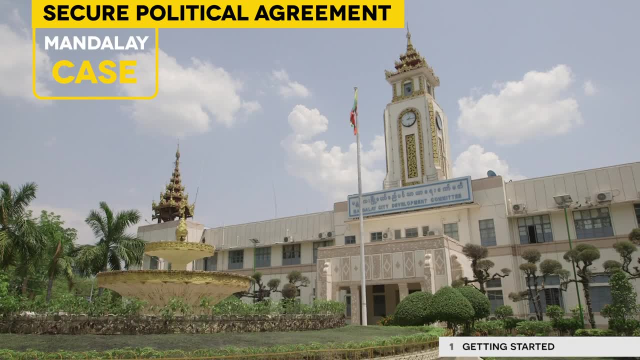 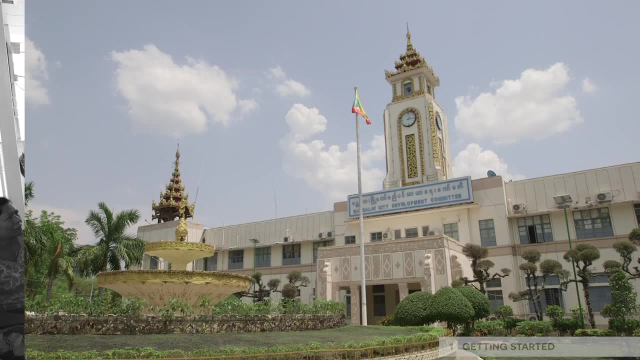 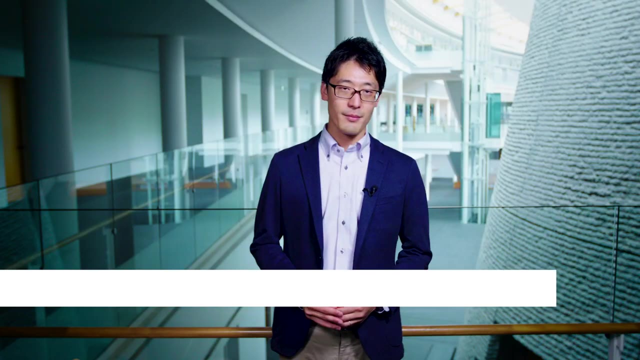 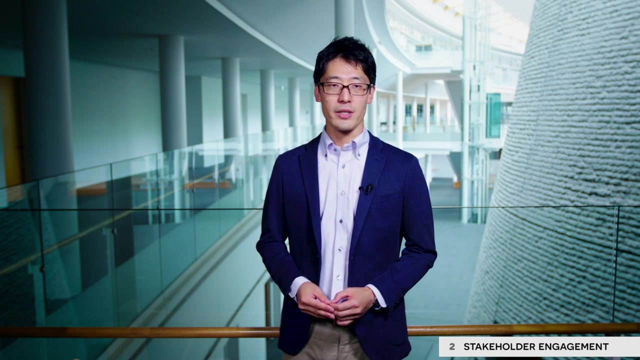 In this way, the development of the strategy came to be truly owned by the local government agencies. Step 2. Engaging stakeholders: Identify all interested groups. Governments will have a leading role in developing any national waste management strategy and agencies with sectoral responsibilities. 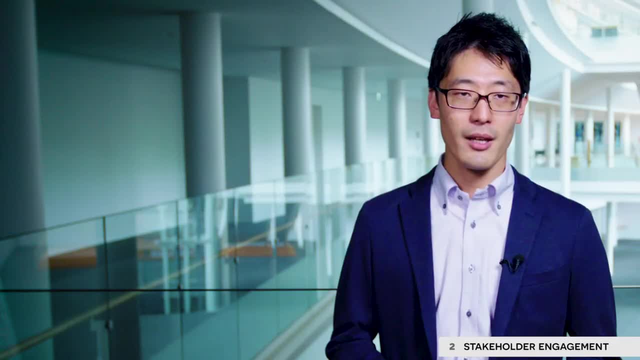 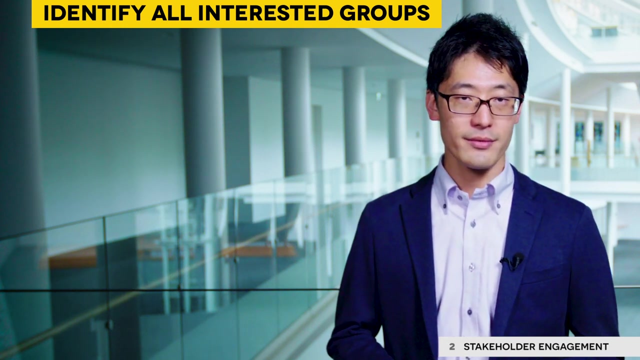 like environment or health, will play key roles. But apart from government agencies, within each country, a great variety of organizations and groups play vital roles in waste management activities, and you must identify all these relevant stakeholders. They fall into one of three categories. 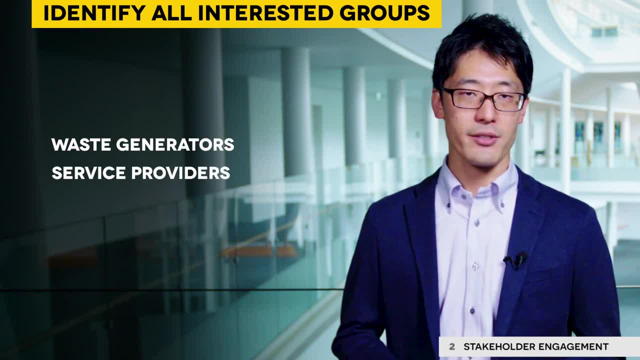 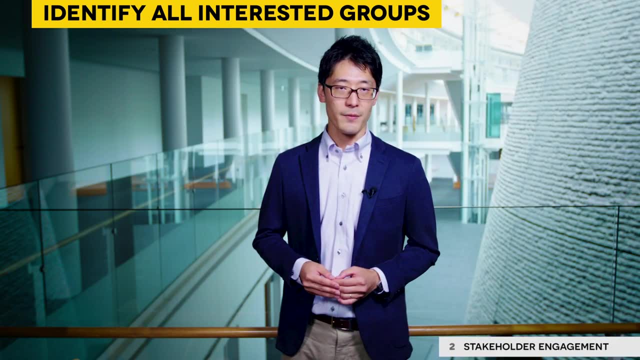 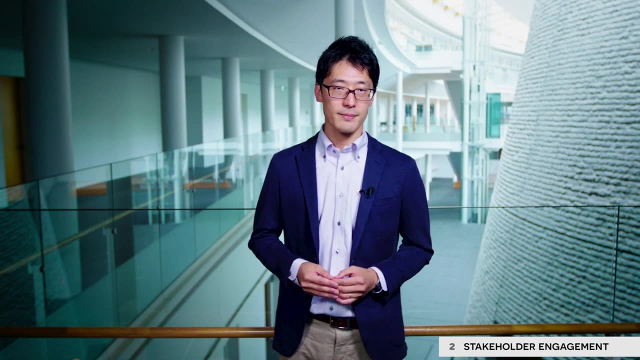 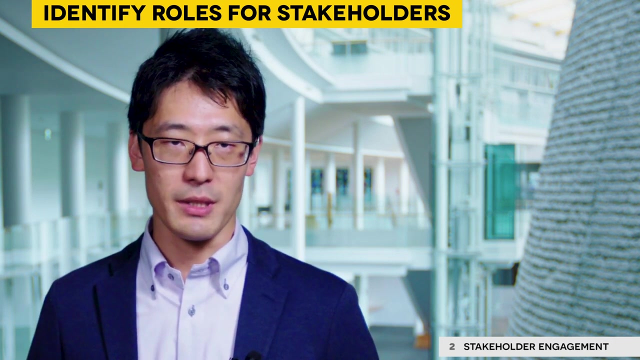 waste generators, service providers and supporting entities. Members of these categories can be found in the community, Private sectors, NGOs, civil society and academia. Identify roles for stakeholders. Identifying the groups that are actively involved in waste management. Getting them involved in the discussion from the beginning. 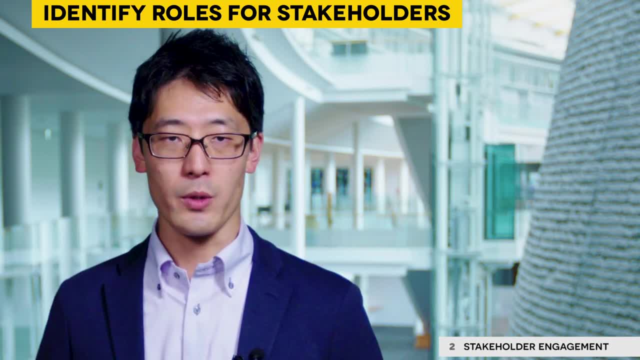 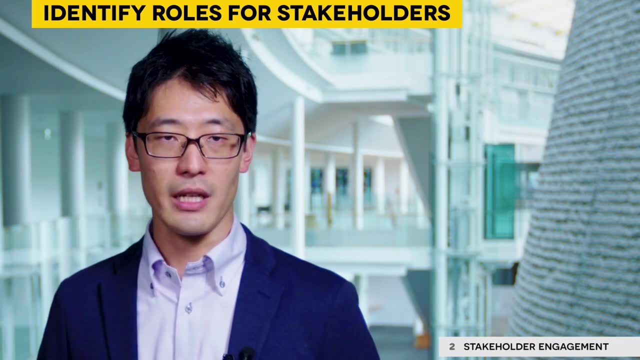 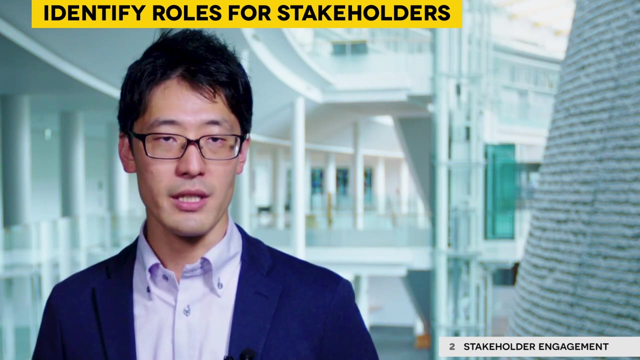 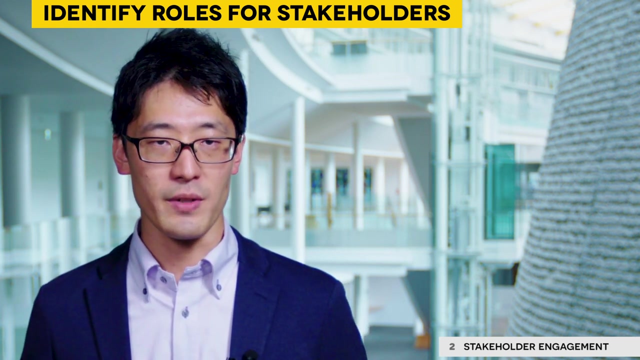 and determining their roles is very important in the development of a sound waste management strategy. Different stakeholders can support the initiative in unique ways. NGOs, for example, often have experience working with communities at the grassroots level and can play an instrumental role in complementing the waste management service provided by the government. 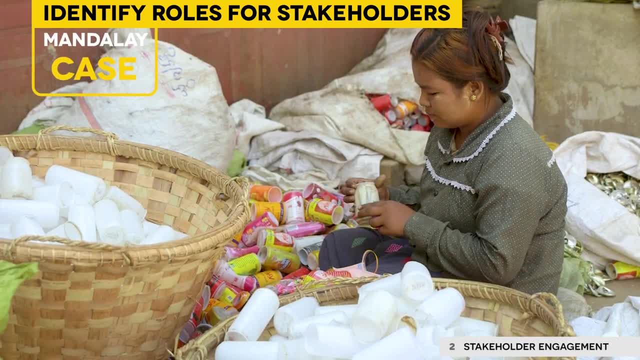 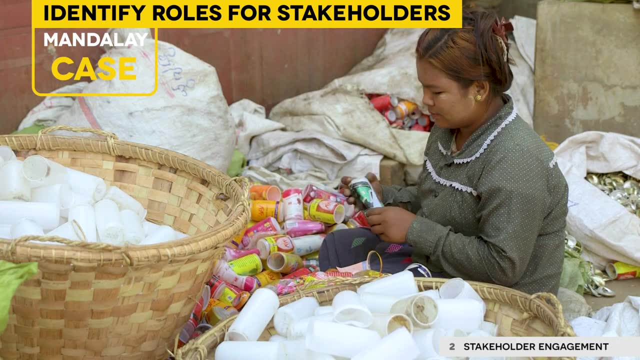 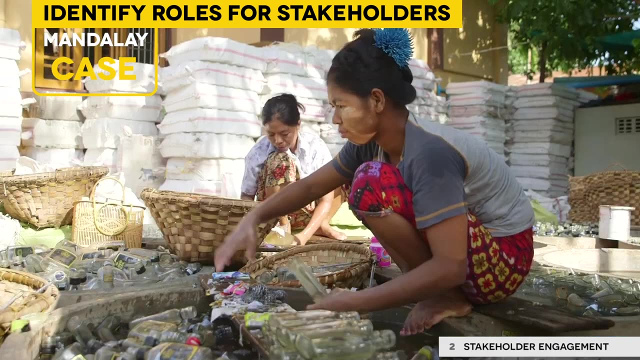 In the case of Mandalay, there are already a lot of informal waste recyclers collecting materials from households and selling them for profit. We consider them to be very important stakeholders, As they could support recycling activities in the future, so we involve them in the development of the waste management strategy. 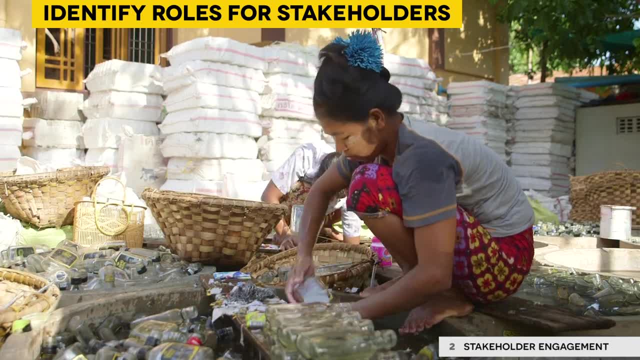 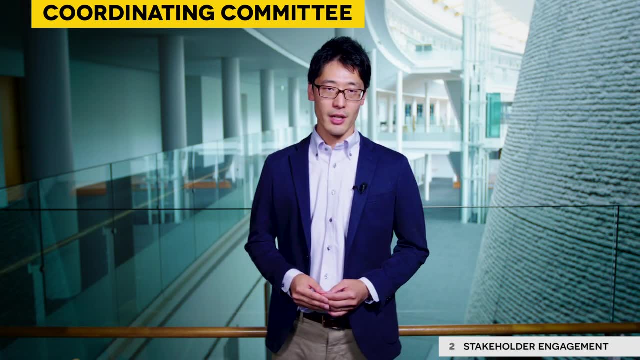 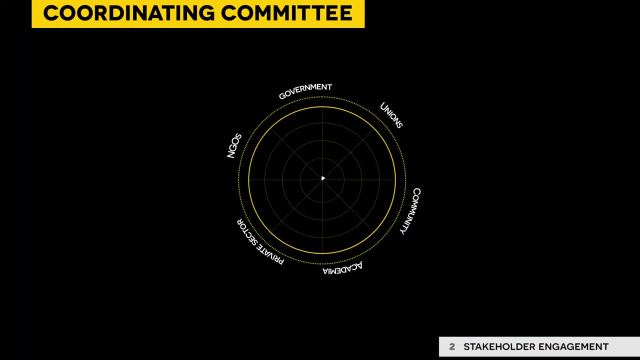 from the very beginning with other stakeholders. Establish a coordinating committee To organize the involvement of all these stakeholders. a working committee should be established to provide coordination of the project activities. The committee should be formed by representatives from different stakeholder groups so that they can all participate in the discussions. 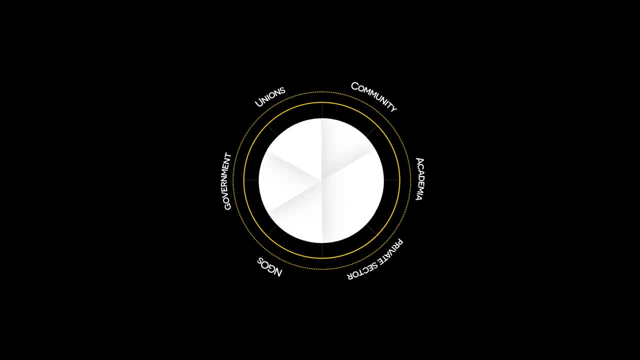 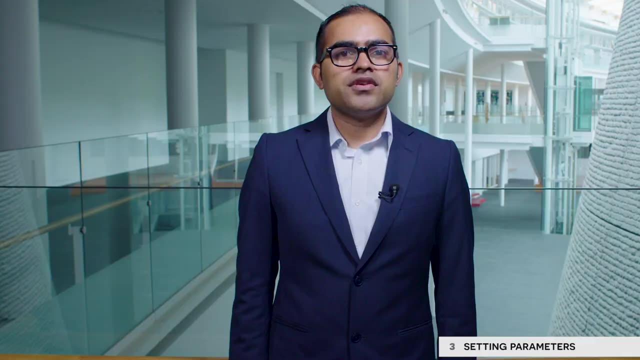 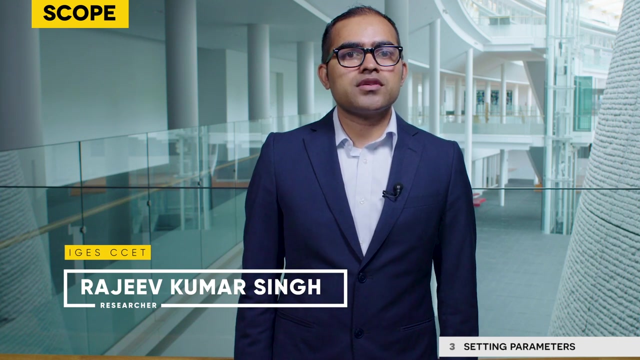 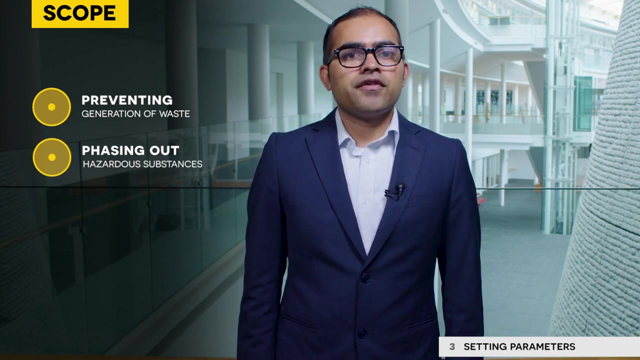 throughout the strategy development process: Step 3. Setting parameters. The general dimensions, focus and scope of the strategy should be decided early. The strategy should focus on preventing the generation of waste and phasing out the use of hazardous substances in the products, rather than simply on managing. 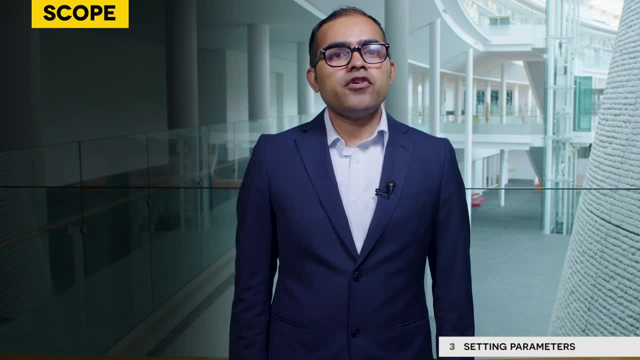 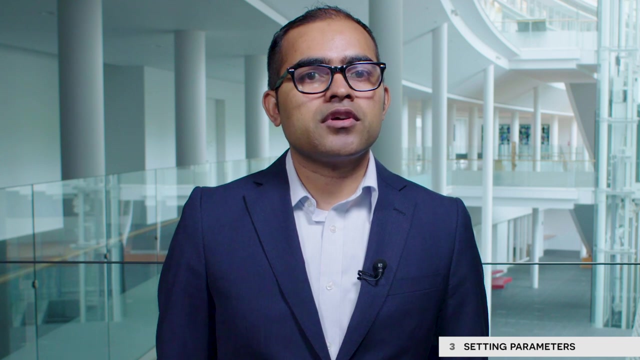 what is generated. While some categories of waste may be allocated a higher priority initially, any waste stream, even if it is of minor significance at present, will need to be managed at some stage. Participants will need to come to a common agreement on the overall vision and mission for this process. 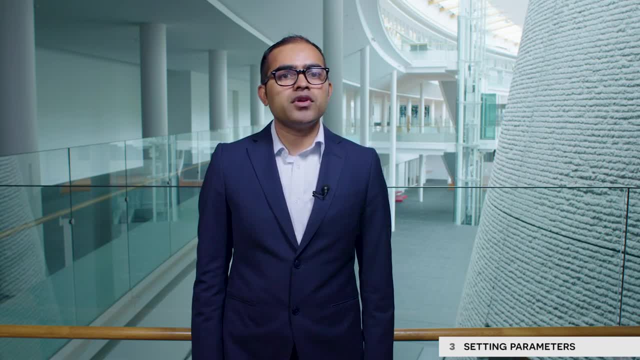 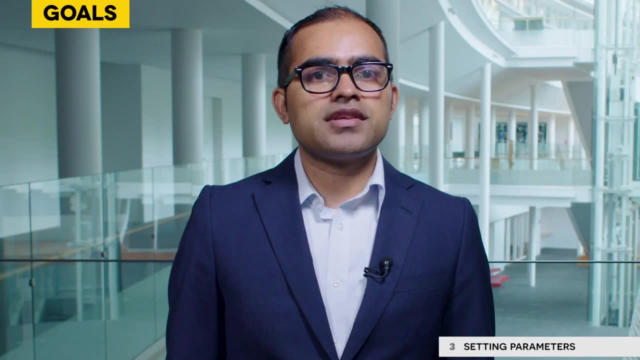 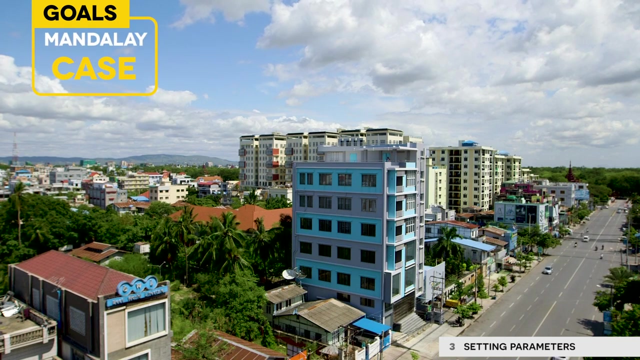 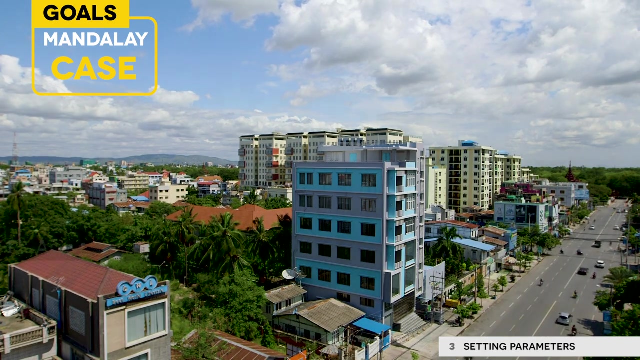 Based on this shared understanding, it is important to identify the major goals. Goals should be accompanied by concrete targets and timetables to measure progress against. In Mandalay's case, the City Waste Management Strategy identifies six goals: 1. Accelerate waste collection and 3R activities. 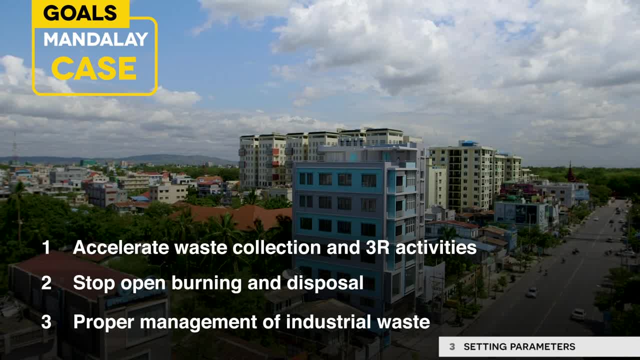 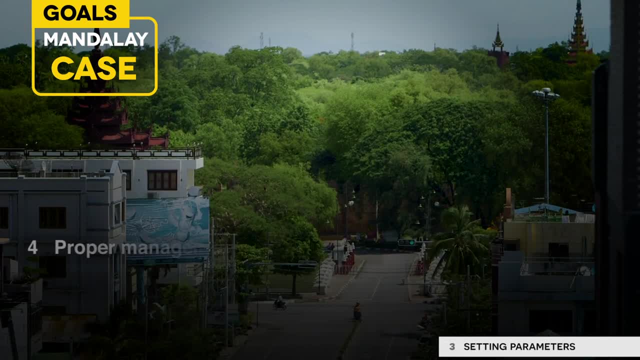 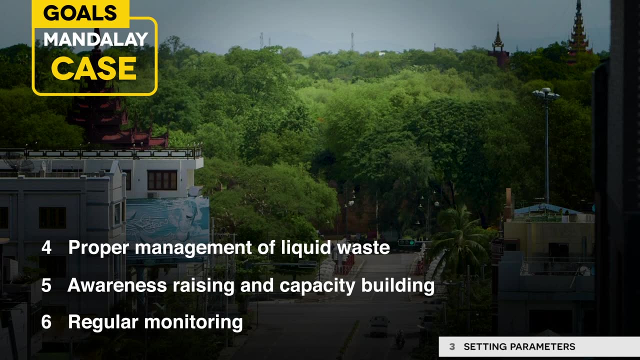 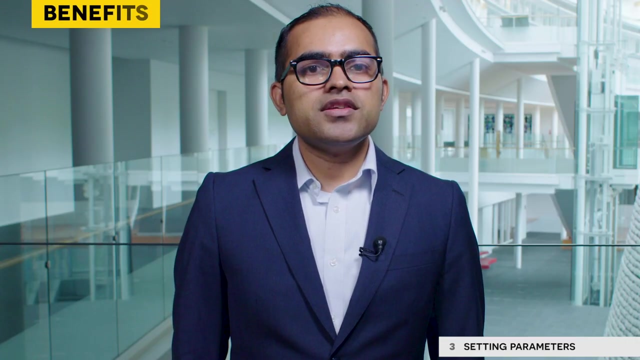 2. Stop open burning and disposal. 3. Proper management of industrial and other waste. 4. Proper management of liquid waste. 5. Awareness raising and capacity building. 6. Regular monitoring. The strategy process should highlight the benefits. 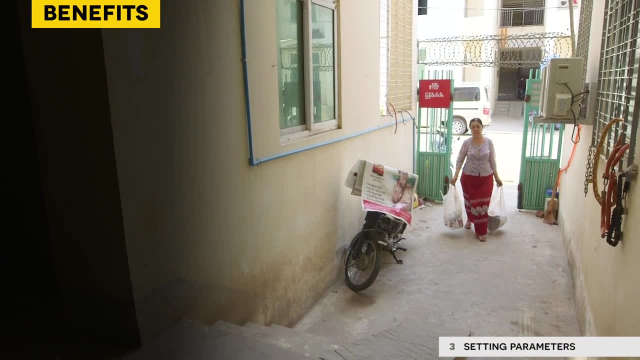 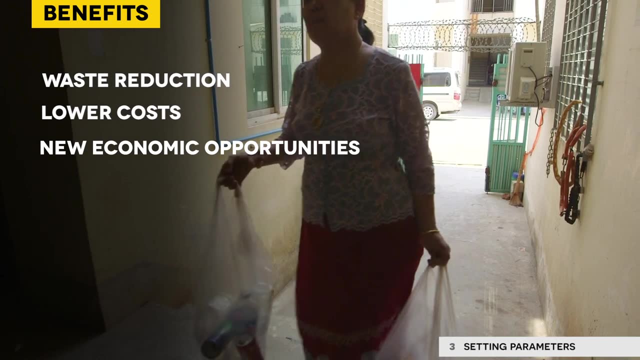 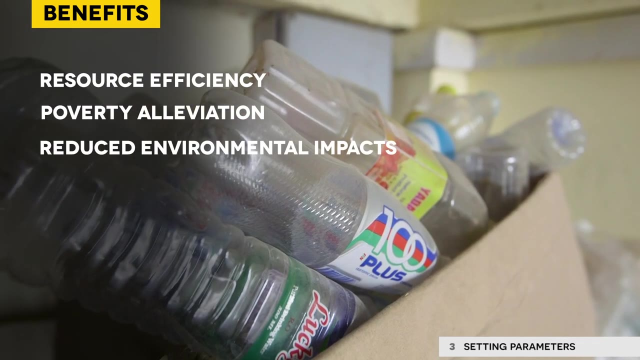 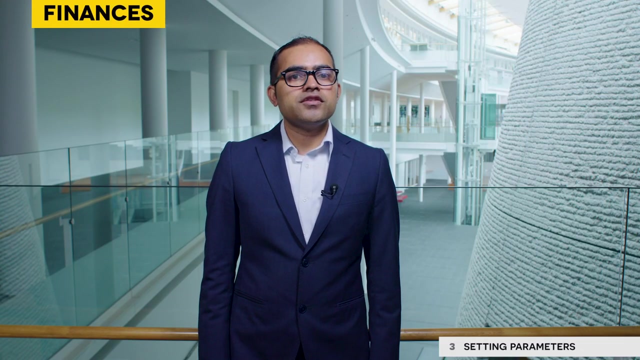 of better waste management. These include waste reduction, lowering operating cost, new economic opportunities, resource efficiency, poverty alleviation, reduced environmental impacts and improved health. Secure adequate finances and other resources for strategy development. to ensure that development does not stop, The capacity is necessary to undertake. 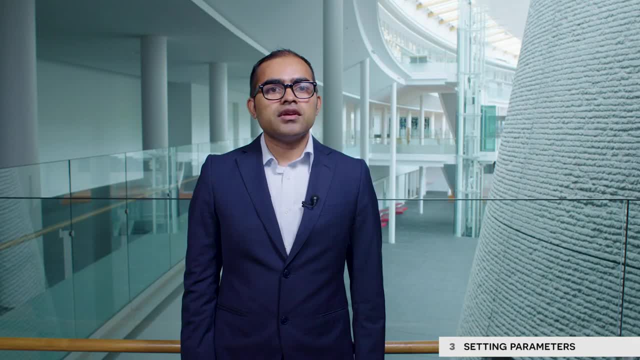 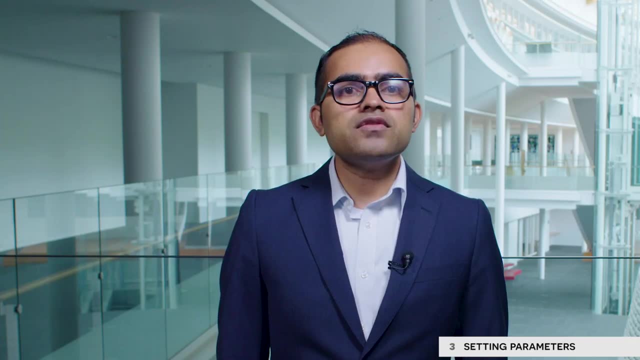 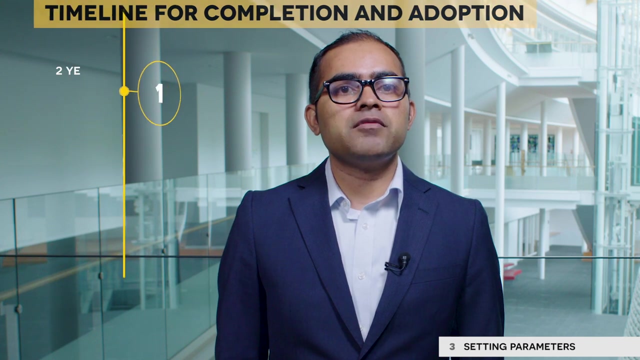 the strategy need to be considered. For instance, a country with limited capacities available may choose to limit the scope in the initial stages. It is important to have a clear timeline for strategy completion and adoption and include milestones over the term of 2,, 5, and 10 to 20 years. 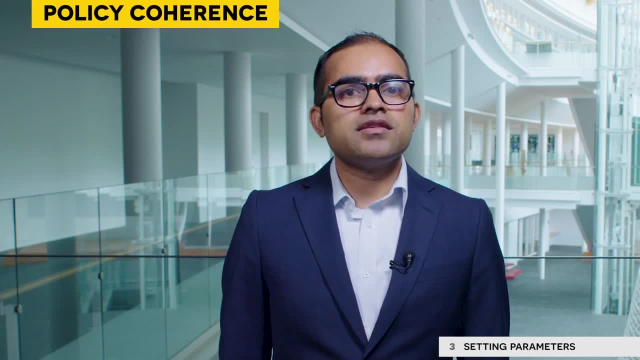 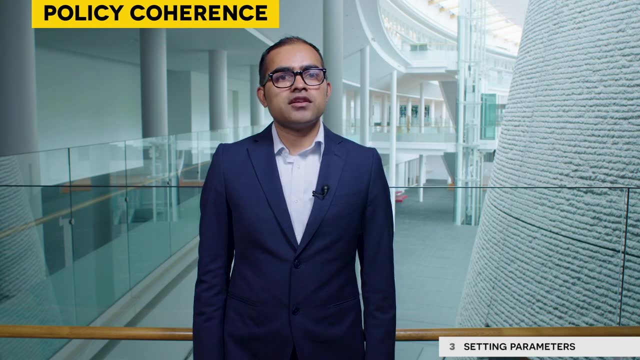 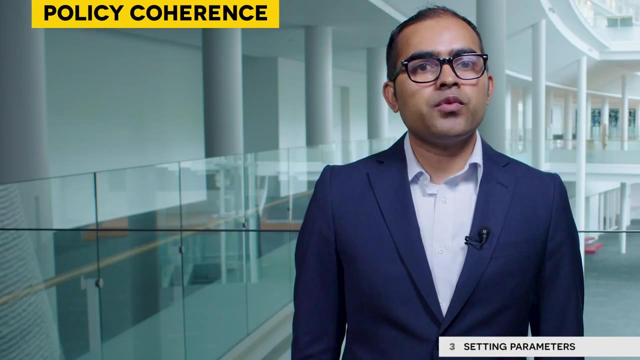 Policy coherence. The potential interaction of waste management strategy with other policies need to be considered. Positive interactions are to be encouraged to ensure that the waste management strategy can be implemented in the best way possible. In addition, the waste management strategy will need to be resolved. 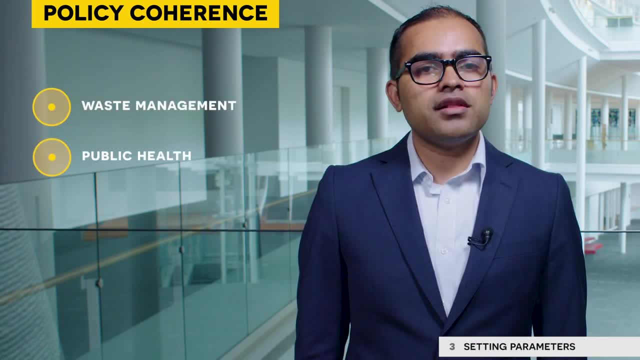 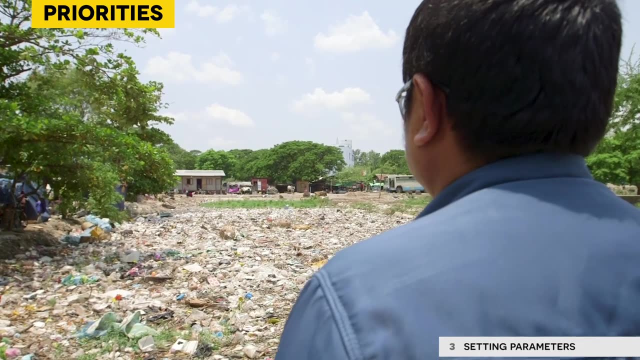 Consider whether the waste management strategy would be linked to existing plans for municipal waste management, public health, environment or urban development. You must set priorities as to how and when you deal with different kinds of waste. You may have to urgently address waste streams. 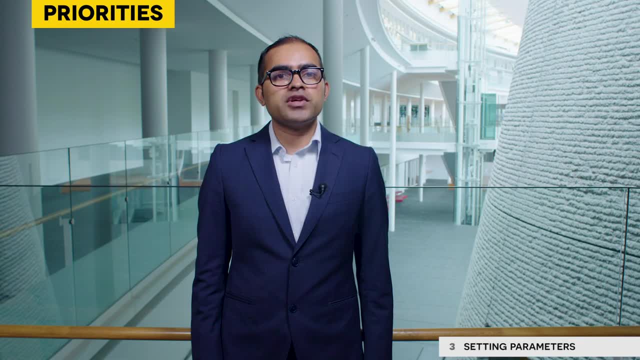 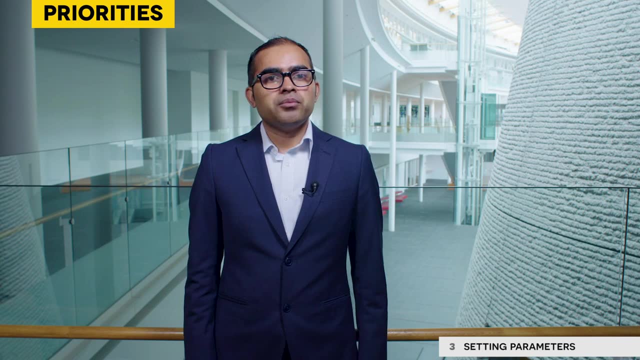 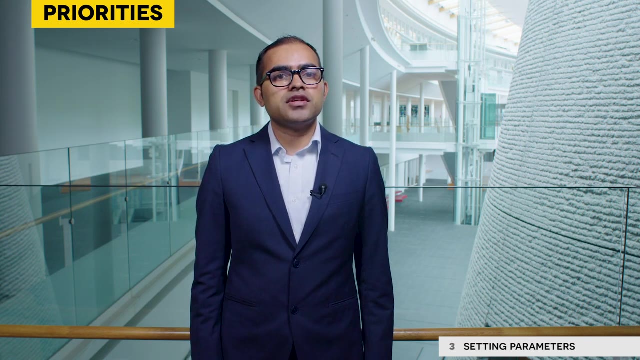 that are especially problematic. Most countries will have several waste management priorities which need urgent attention. while other waste streams will be addressed later, Municipal solid waste management will be a priority for any city, because the provision of these services is key to keeping the city operating. 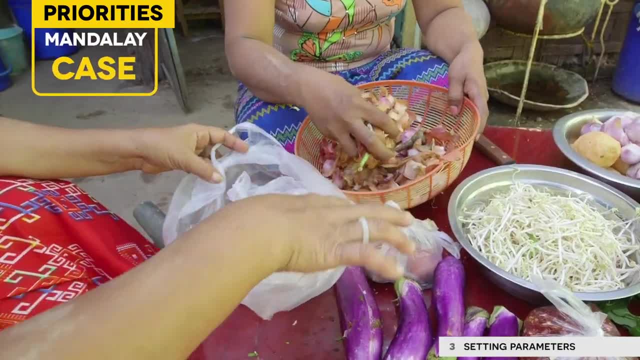 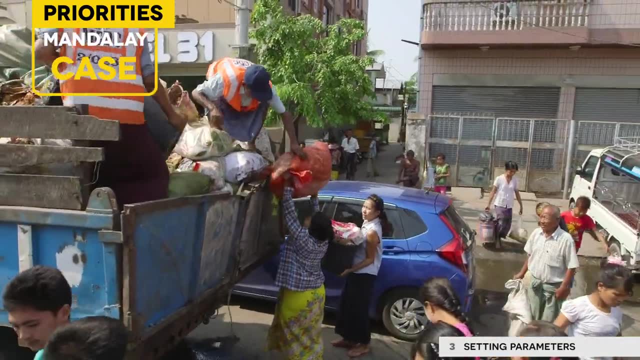 In Mandalay's case, following the assessment, they prioritized the municipal waste issue because it was within the mandate of the cleaning department, the leading agency in the development of waste management strategy, While they concluded it was important to deal with hazardous and industrial waste. 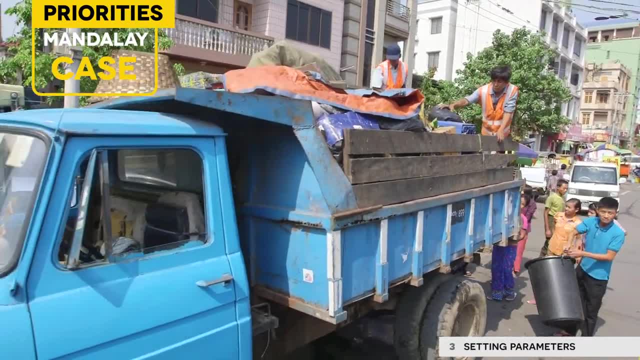 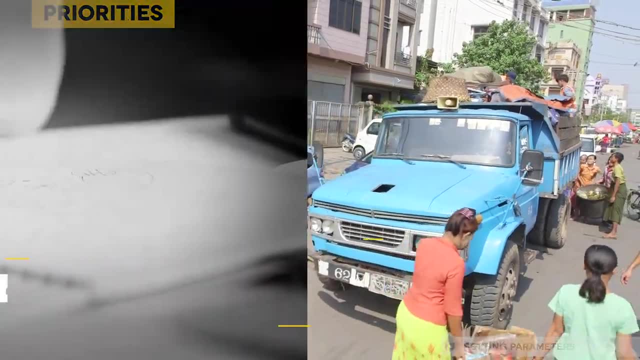 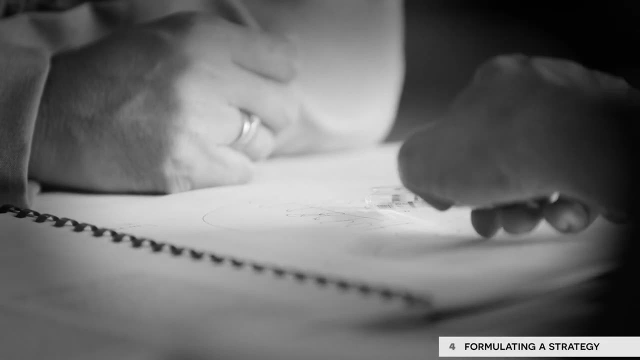 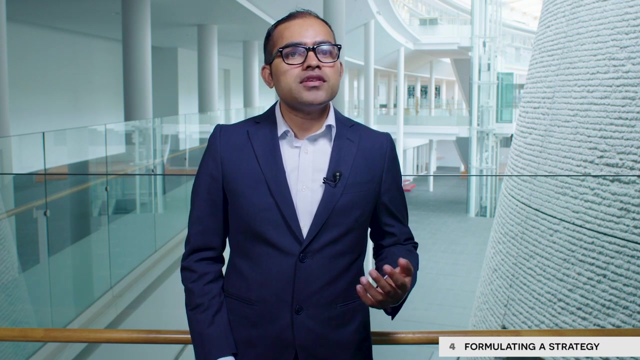 this required the cooperation of more government agencies, making implementation more complicated, so they decided to tackle this later. Now that you have reached a common understanding of the parameters for the strategy, it is time to start drafting the actual strategy. It is important to consider each issue's. 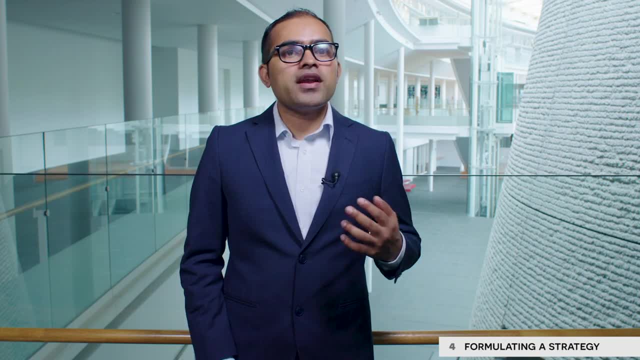 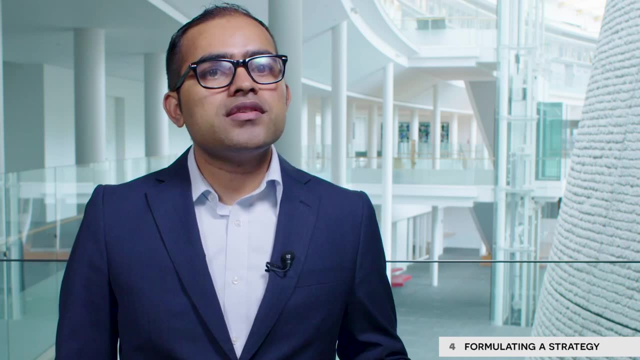 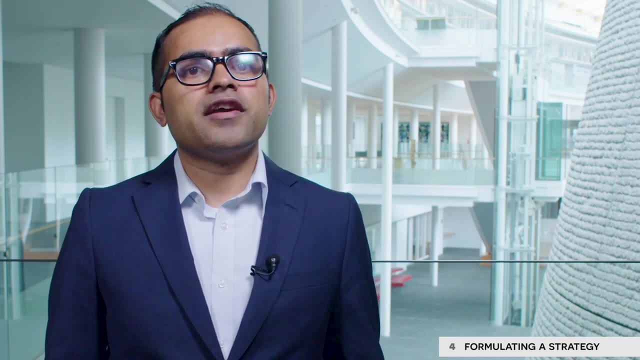 identify in a previous step and what actions can be taken to address it, based on the goal set. How is the issue managed at the present? What are the opportunities for the waste prevention, materials, recovery and recycling? What policy options are available to address this issue? 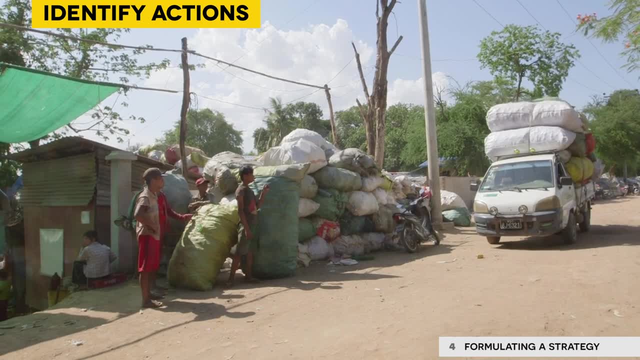 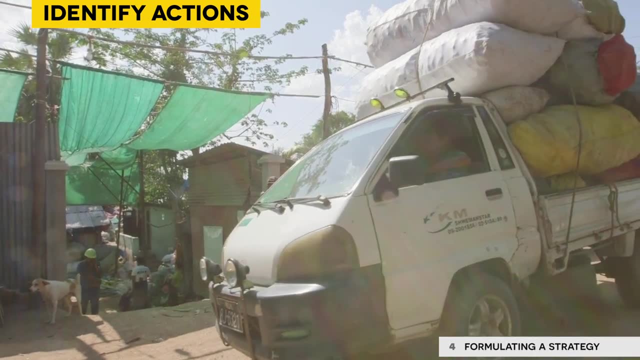 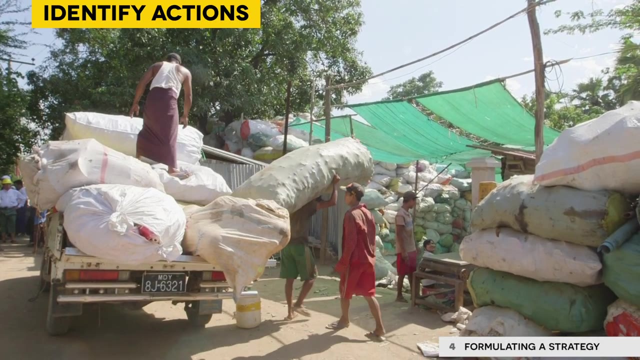 Identify actions. Choices about the management of each waste stream or issue should be carefully analyzed. The aim is not to manage waste better or to ensure compliance with regulations, but rather to optimize the use of limited material resources. This means avoiding the generation of waste at the source. 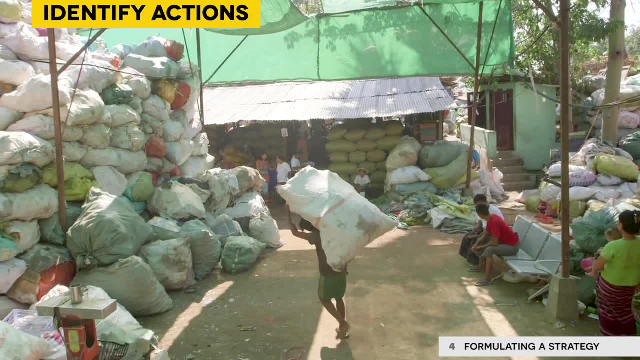 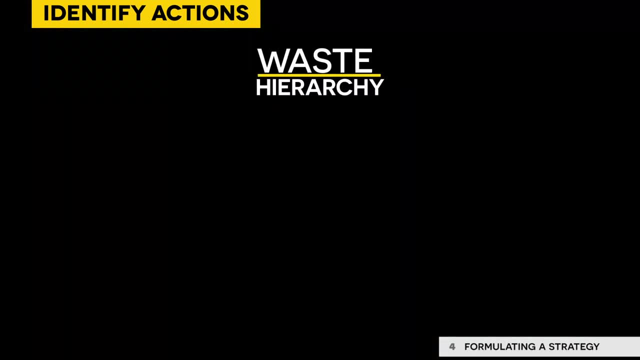 by treating it as a resource waiting to be recovered and reused. Discussions should be guided by the waste hierarchy, which indicates an order of reference for actions to reduce and manage waste. The hierarchy illustrates a prioritization of action for waste management activities, giving top priority to preventing the waste. 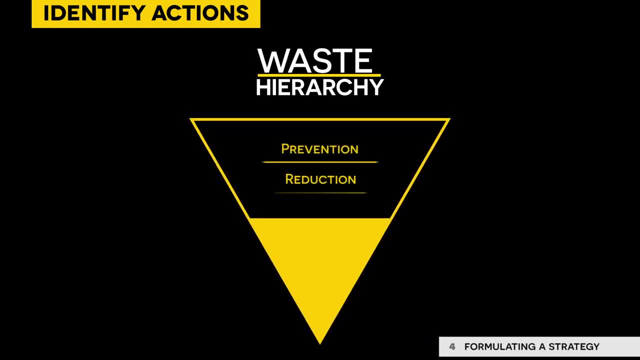 from being generated in the first place, followed by reduction through means such as reuse, recycling, recovering of energy through waste processing such as anaerobic digestion, incineration and so on, and finally disposal at last resort, Once action has been identified. 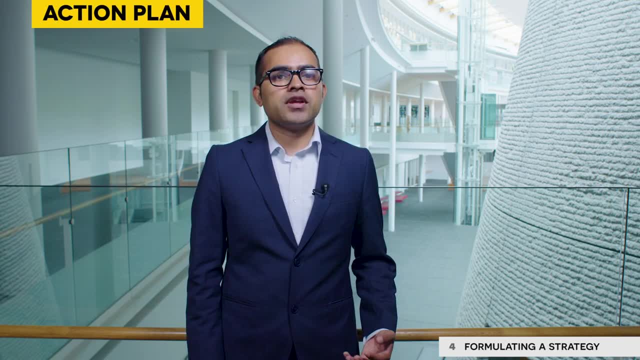 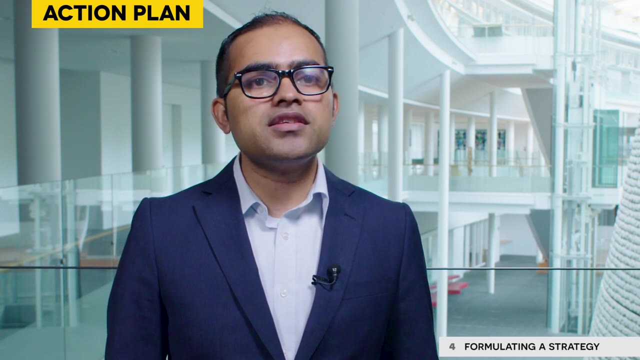 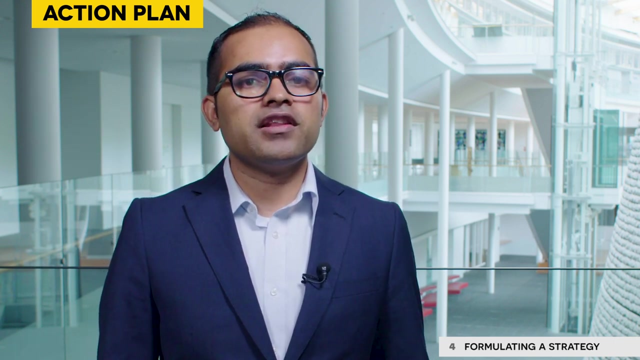 an action plan should be prepared for each waste stream or issue, with accurate budgets and the responsibilities for implementation clearly identified. Necessary policy instruments identified in these action plans will need to be integrated in existing laws and regulations through appropriate amendments, or new laws and regulations introduced, whether relevant. 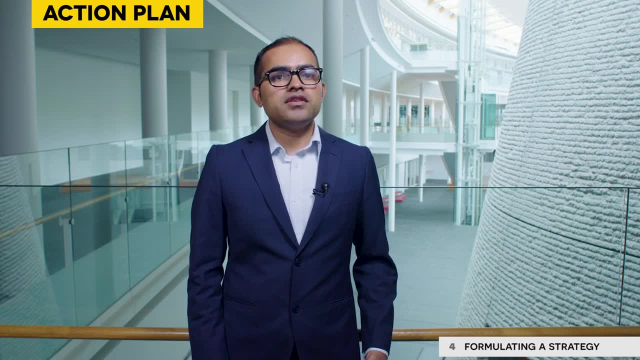 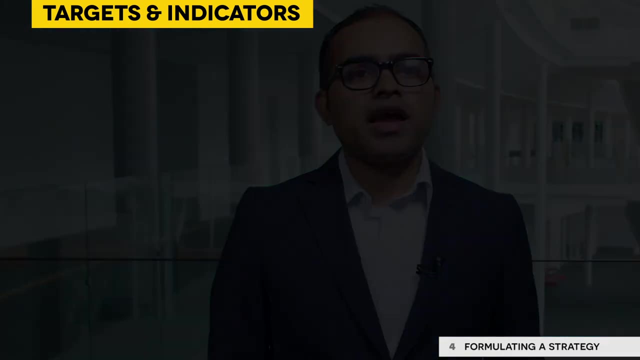 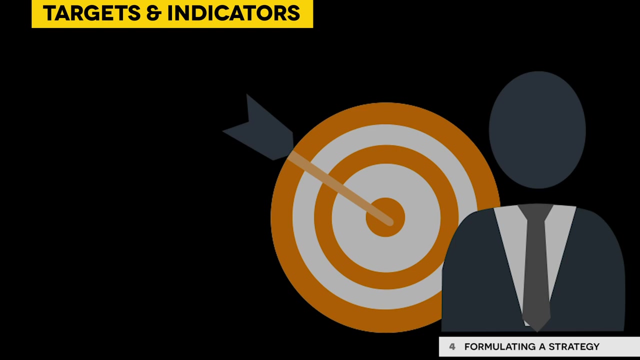 We recommend that you identify initial actions that can be easily implemented, so the partners can start working together and achieve early results. Establish targets and indicators In developing the action plans. targets should be set for priority waste streams or other issues, for example, reduction of waste generation. 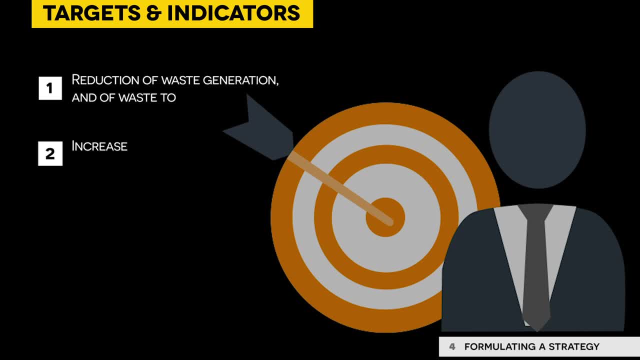 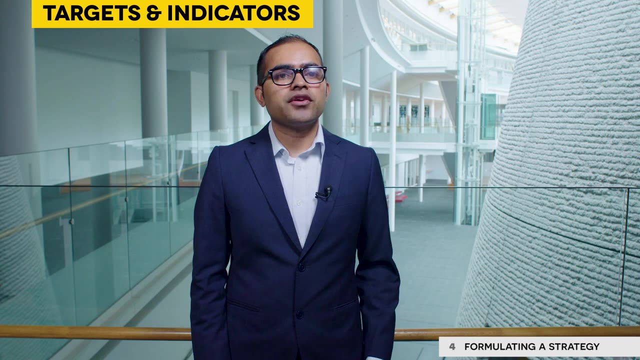 and of waste to be landfill. increased waste collection rate or coverage and increased recycling rate. targets for moving from uncontrolled dump sites to properly engineered landfills. These targets can be used to drive actions, create momentum, monitor progress and alert those implementing. 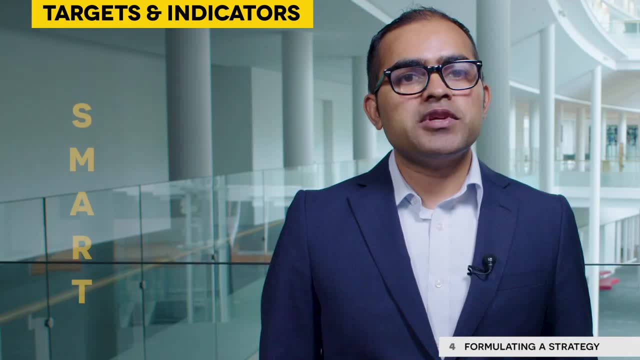 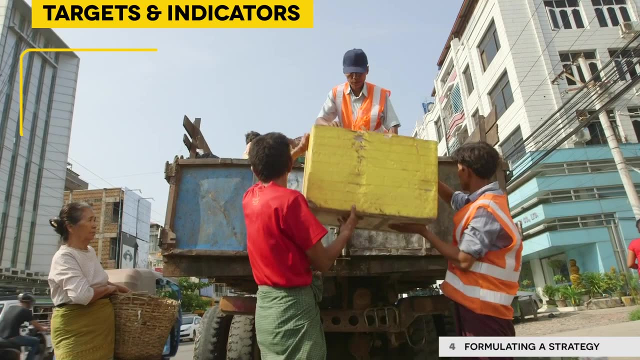 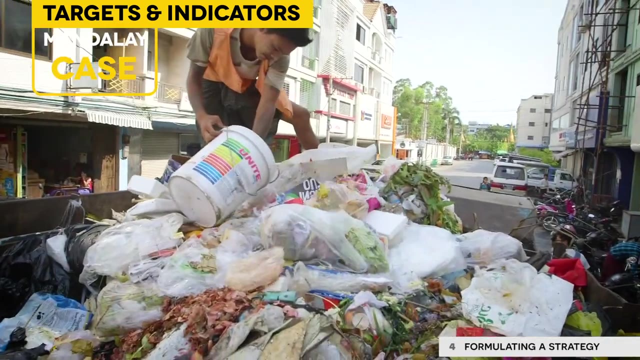 the strategy to problems. Targets should be smart, specific, measurable, achievable, relevant, time-bound. In the case of Mendeley, stakeholders decided as a first goal the improvement of the waste collection service in the city. Currently, it covers 70% of the city. 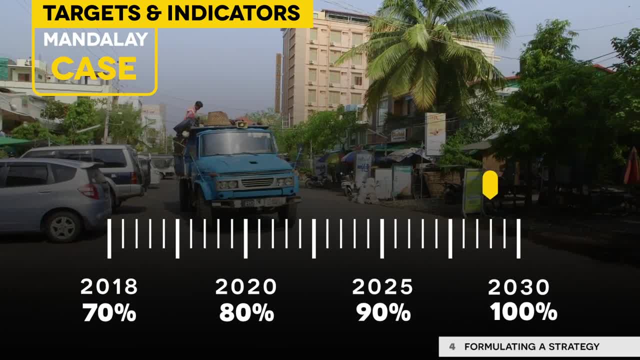 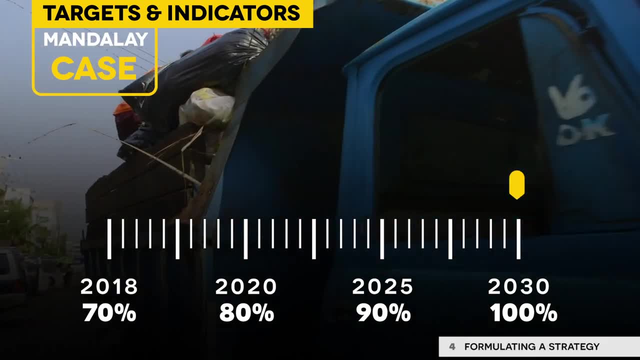 Their target is to provide 100% waste collection service in the city by 2030.. They also defined some mid-term targets: 80% by 2020 and 90% by 2025.. As you can see, targets are time-bound. 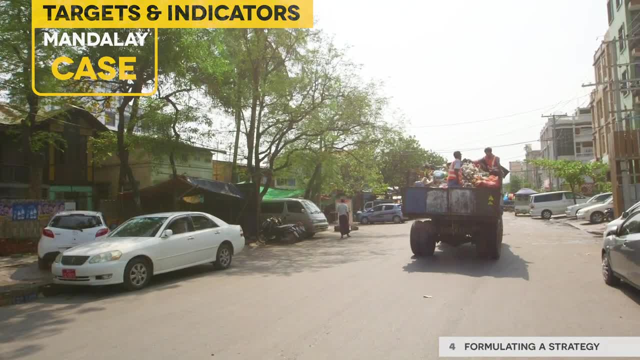 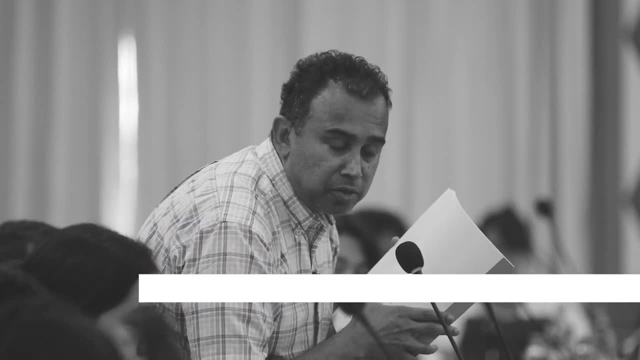 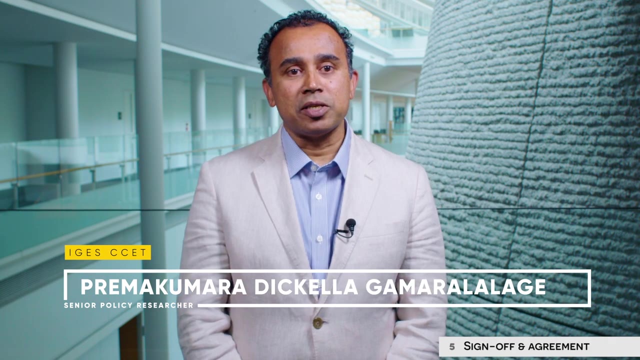 They help monitor progress in waste management. Step 5. Sign off an agreement Once the actions have been drafted. the strategy is practically completed. It is important, though, that the strategy is officially endorsed by the public and government officials. The strategy should be submitted. 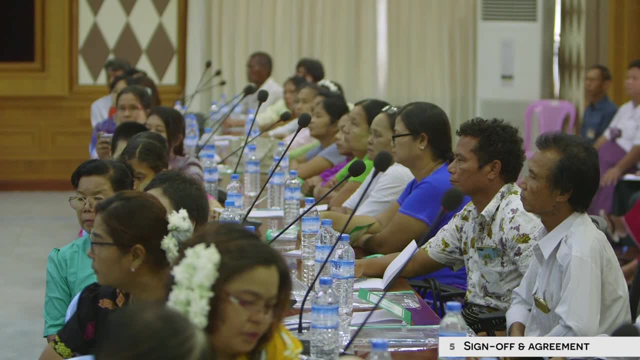 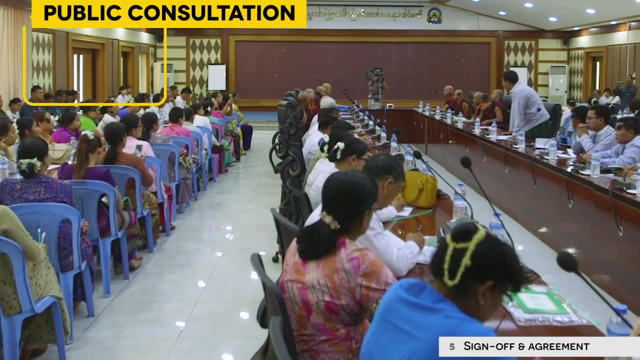 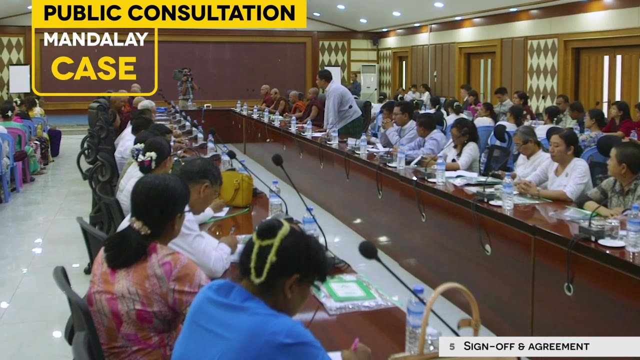 to a full public consultation process in which the public is invited to provide feedback. In the Mendeley case, after the strategy was completed they organized a large public meeting to present the waste management strategy to various stakeholders. They listened to their concerns and achieved commitment to implementation. 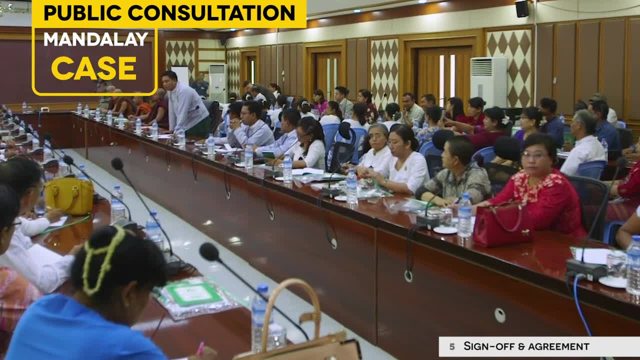 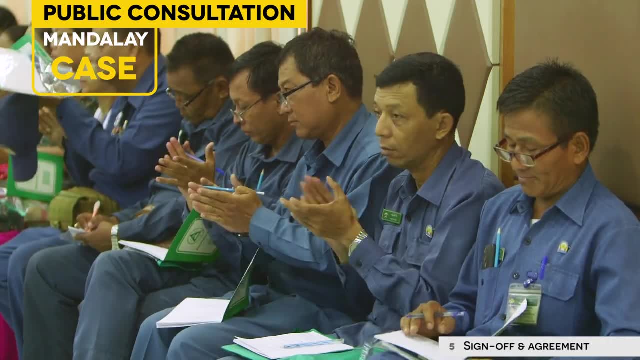 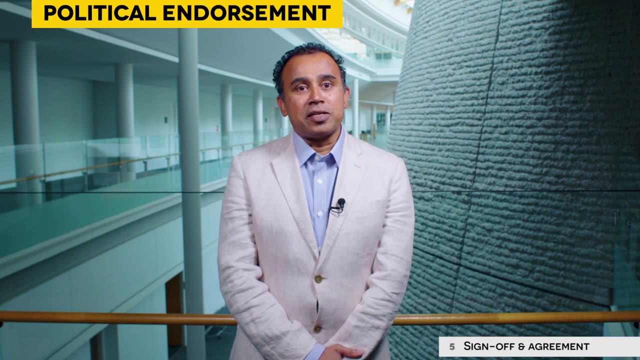 News of the strategy also appeared in the media. The strategy document was distributed among people dealing with waste management. The final step in strategy development is political sign-off and getting approval. This endorsement is crucial during implementation to secure budget and staff allocated to improving waste management. 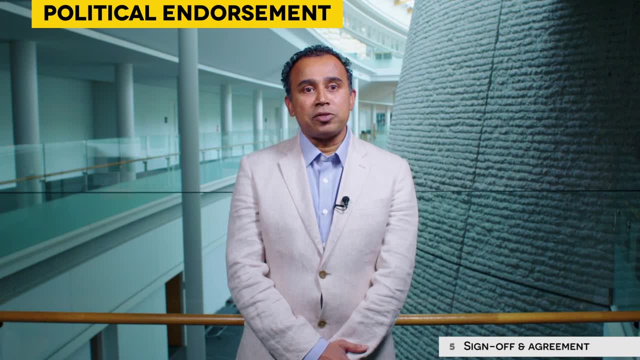 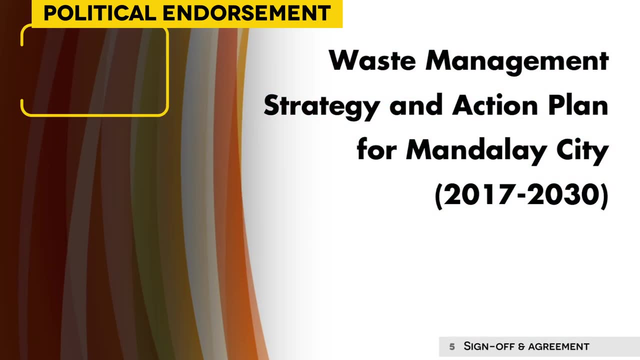 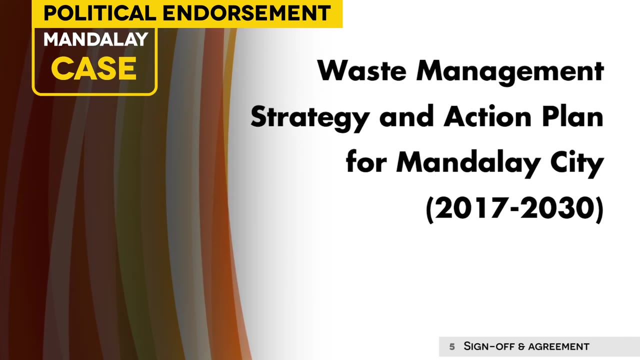 In the Mendeley case, the strategy was distributed to various stakeholders. The strategy was distributed to various stakeholders. This endorsement is crucial during implementation to secure budget and staff allocated to improving waste management. In the case of Mendeley, after the final workshop: 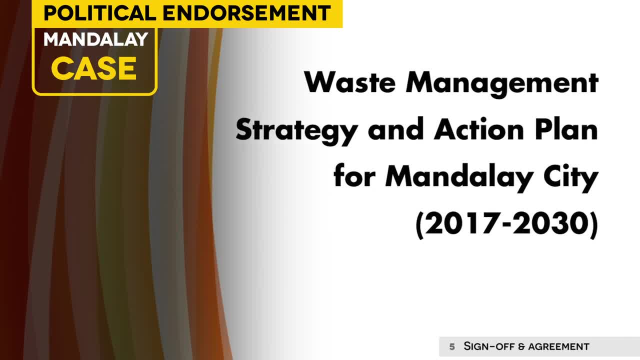 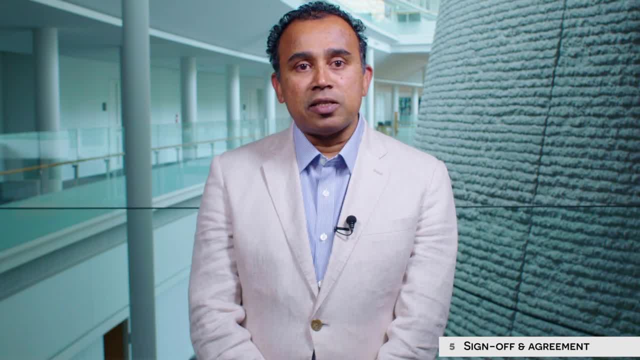 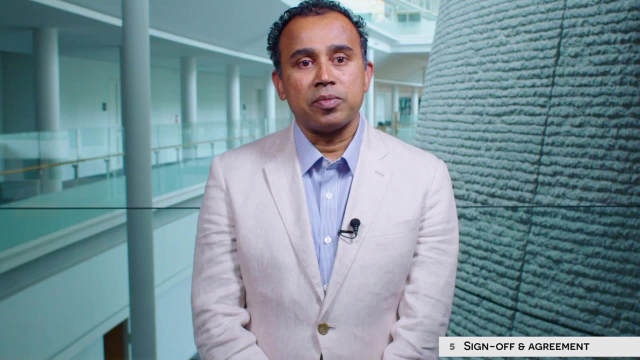 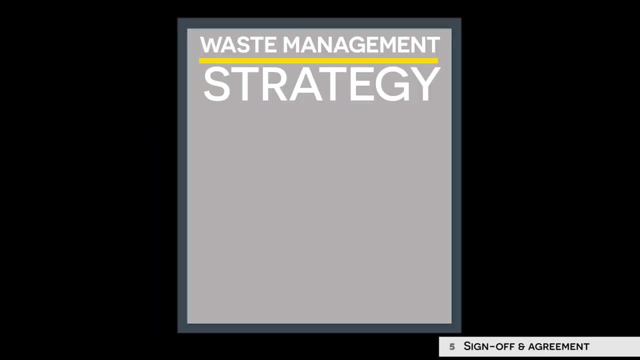 they submitted a report to the City Development Committee for official approval. They also got approval from the regional government to make their legal document for their next ten years as a printed and digital publication. The outcome of the process is a waste management strategy consisting of a number of elements: An ambitious overall framework and goals for sound waste. 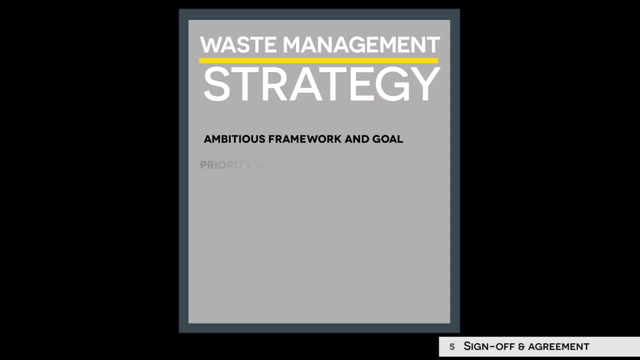 management in the city or country. A list of priority waste streams and issues. An action plan for each waste stream or issue comprising one or more targets and policy actions. Cost estimates for each action plan. Clearly allocated responsibilities for implementing the actions identified. Plans for review, including indicators to measure progress and collection of appropriate. 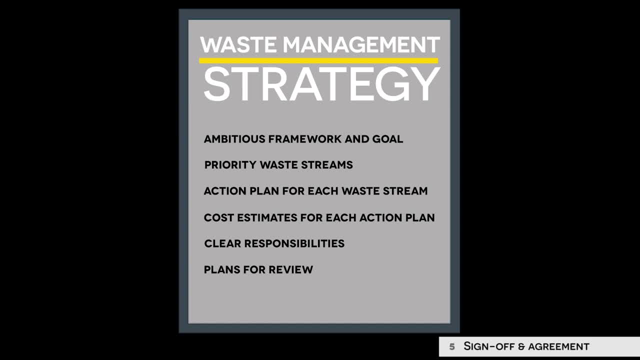 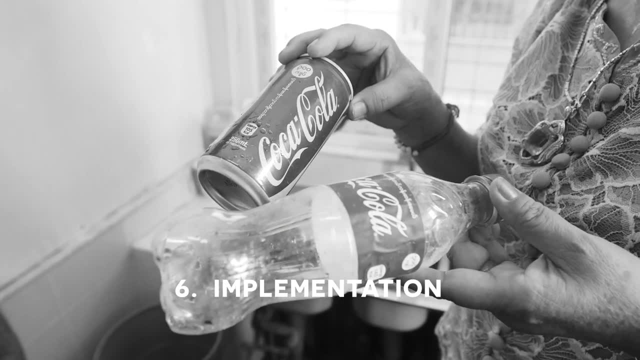 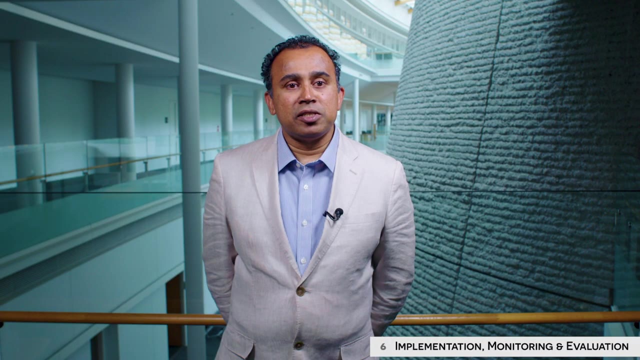 data and revision of the strategy on a regular basis and as developments require. Step six: implementation, monitoring and evaluation. This step is the most commonly overlooked, but it is crucial for success. The waste management strategy should be implemented as planned by the responsible parties. Monitoring: 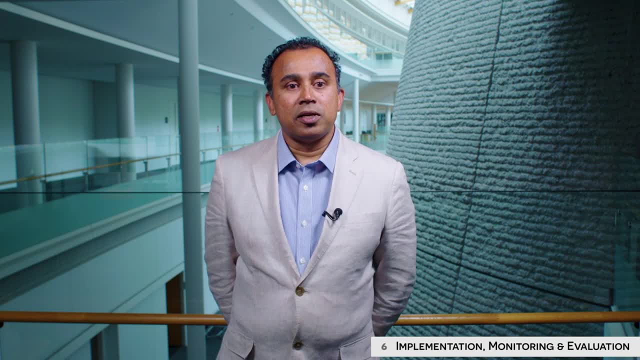 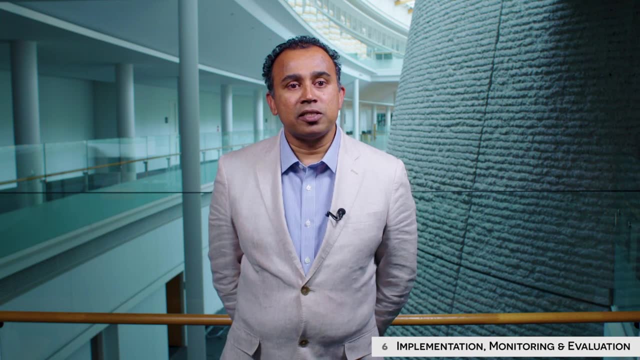 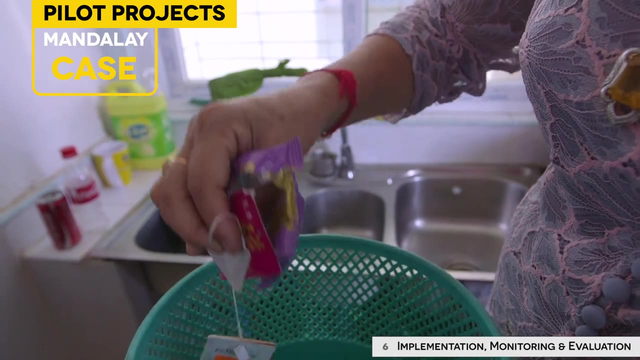 of the targets and indicators is crucial. Based on the result of this monitoring, adjustments need to be made regularly to ensure the strategy is effectively leading to the agreed goals. Mandalay City has implemented some pilot projects for waste separation in households, linking them with entities specializing in recycling. 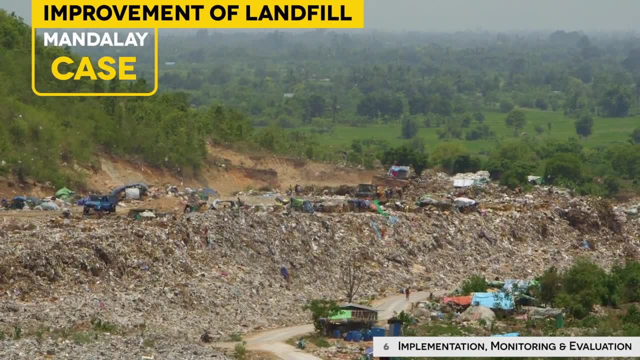 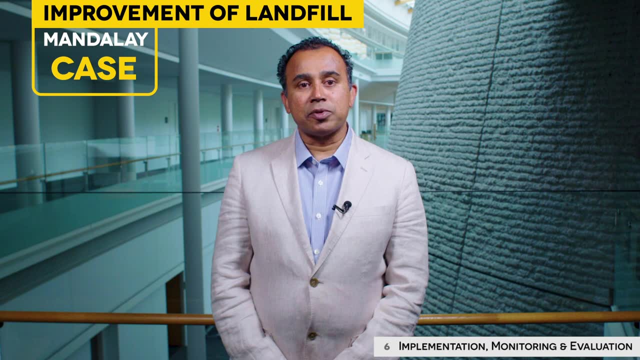 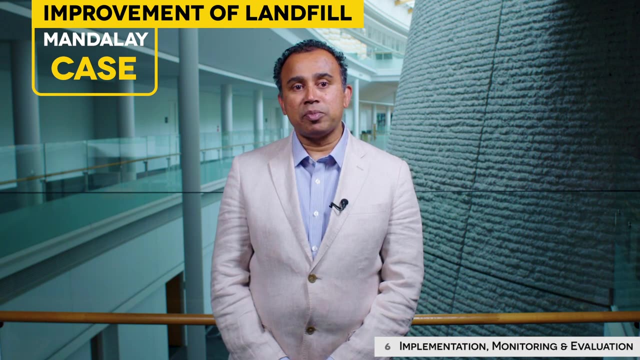 Implementation has now moved to the improvement of the landfill and budget has been secured. This strategy has also promoted external support from Japan to provide an anaerobic digester for managing organic waste, as well as Asian Development Bank's support in improvements of waste management. in line with this strategy, Local partners like Mandalay University and